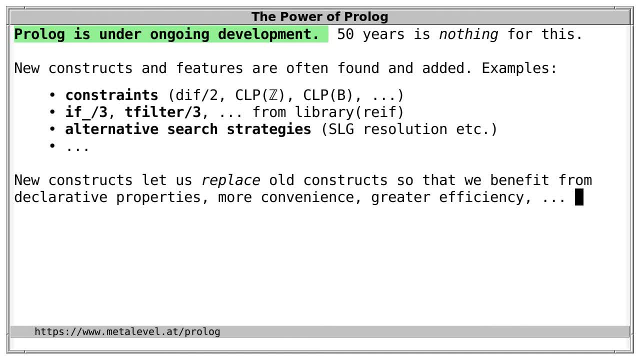 or from greater efficiency and so on. So an important point here is that a few old constructs are now no longer needed, because they are superseded by newer and better features, But for backwards compatibility with older programs the old constructs are also still. 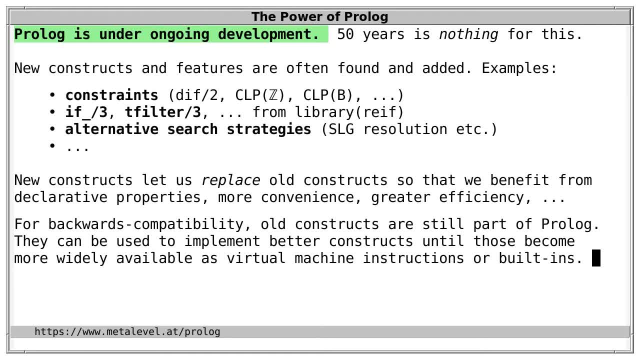 part of prologue, And sometimes we can even implement better constructs in terms of these old constructs, At least until the better constructs become available as dedicated virtual machine instructions or as built-ins. But as a general rule the superseded constructs are of course best avoided in regular programs. So how do we not do it? Well, one thing we 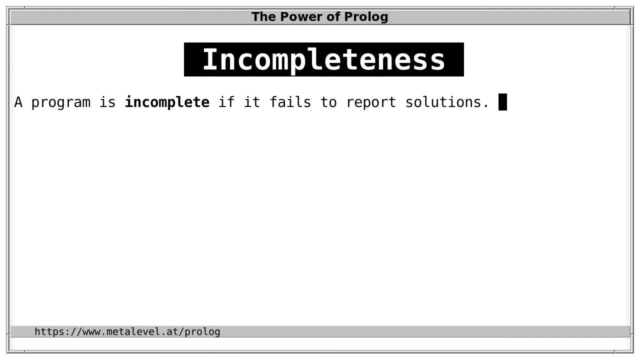 definitely try to avoid is called incompleteness. Incompleteness in the sense that a program fails to report solutions, And it's one thing. if the program is incomplete because it doesn't terminate, That's in a sense okay. A different execution strategy may have better termination properties and be complete. 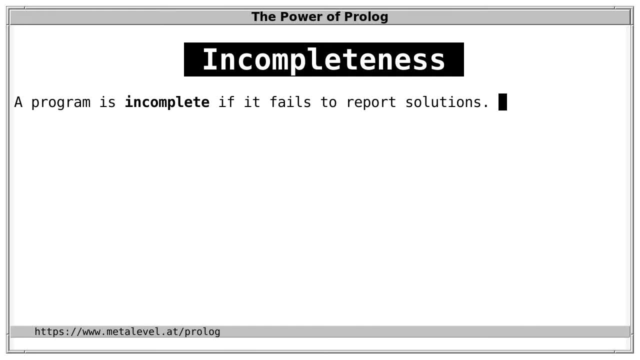 But it's an entirely different thing if the program explicitly tells us there are no or no more solutions, when in fact there are more solutions. That's, of course, extremely problematic, because it's incorrect And there are a few constructs that make our programs incomplete. 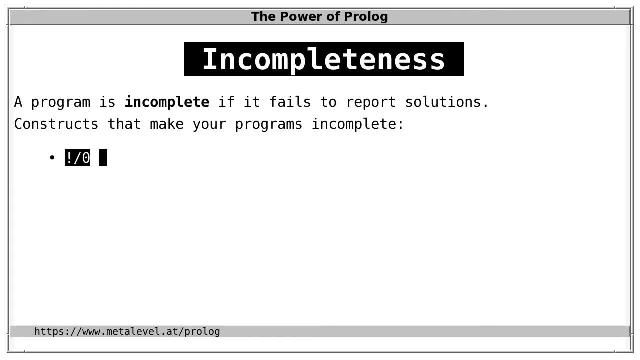 in this latter sense that is incorrect. For instance, this predicate exclamation mark, also called cut, prevents, among other things, the consideration of alternative clauses. So for example, suppose we have a predicate P and we say P holds for the atom A if exclamation mark holds, and P also, and 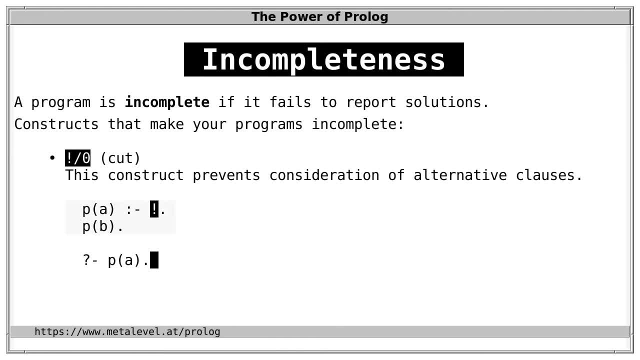 unconditionally holds for B. okay, Then when we query: does P hold for A? Yes, as intended, And does P also hold for B? Yes, also as intended. And now we generalize the query and ask: for which terms X does P hold in general, Then we get A as the only solution And that's clearly. 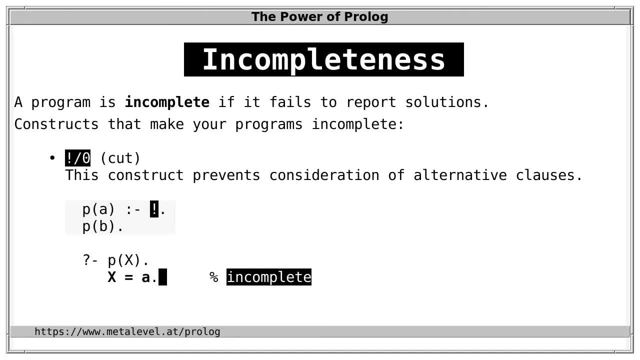 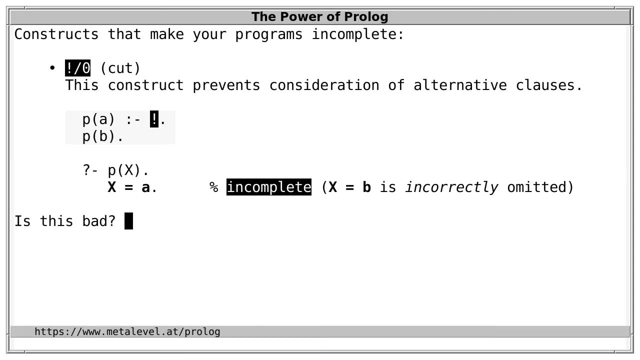 incomplete because we already know that B is a solution too. So in a sense, the predicate has forgotten to mention that there is an alternative, since the solution X is, B is incorrectly omitted. Now one may of course wonder: is this bad? Yes, because important logical properties. 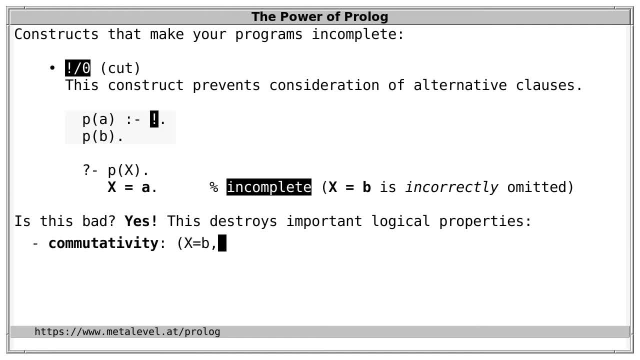 are now destroyed. First, commutativity of conjunction. If you post the constraint X is B before P of X, it yields a solution, because it then succeeds, Whereas if you post the constraint X is B after P of X, that is, we exchange the goals, then it fails And it also destroys monotonicity. 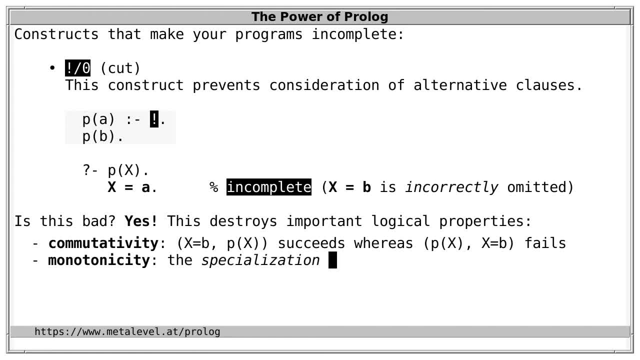 a very closely related property, because the specialization we obtain by adding a constraint X is B, and then we simply state what we stated above. that is, we simply repeat what we said, but we've now added a constraint And remember that the query above failed and we've now. 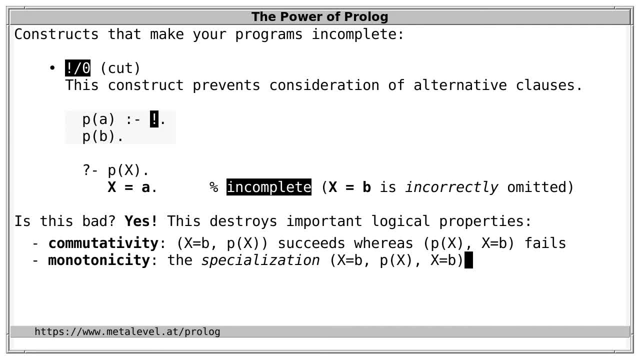 added a further constraint, So we expect it, in a sense, to fail all the more. But no, if we add this constraint, it succeeds. And this is very troubling because it prevents, among other things, alternative execution strategies such as, for example, iterative. 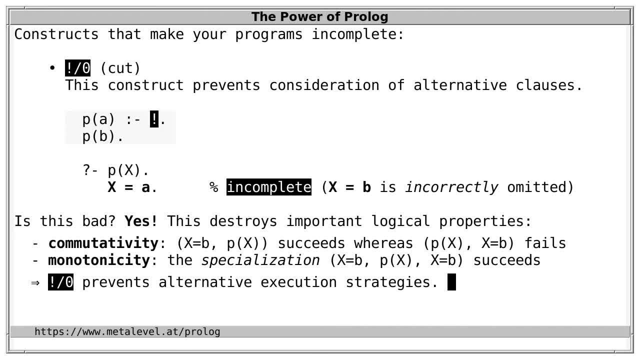 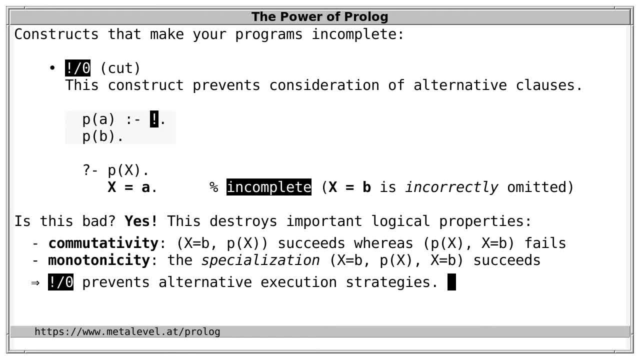 And I mention this because people sometimes blame other predicates, even when they don't destroy these properties Specifically, this is not the problem of the predicate comma, that is of conjunction, Because one could come to the incorrect conclusion here. that comma does not denote conjunction, But it does. It's only that exclamation mark destroys. 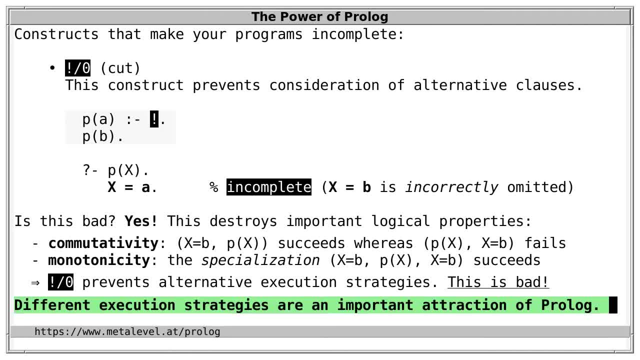 these properties. And yes, this is bad, Because the ability to apply different execution strategies is an important attraction of Prolog. Now one may quickly dismiss this because, truly, who has ever heard of a different execution strategy for Prolog? right That it is something other than depth-first search. 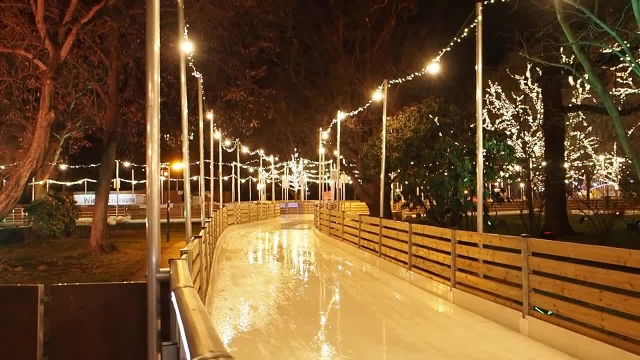 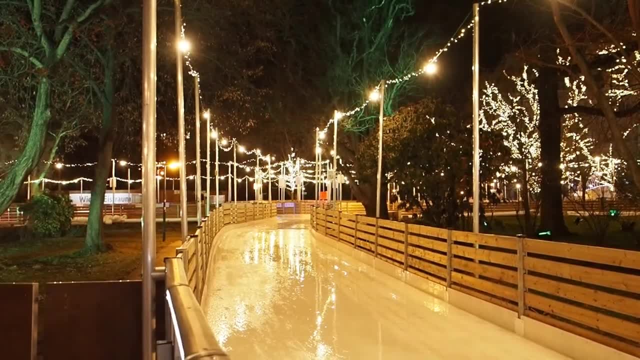 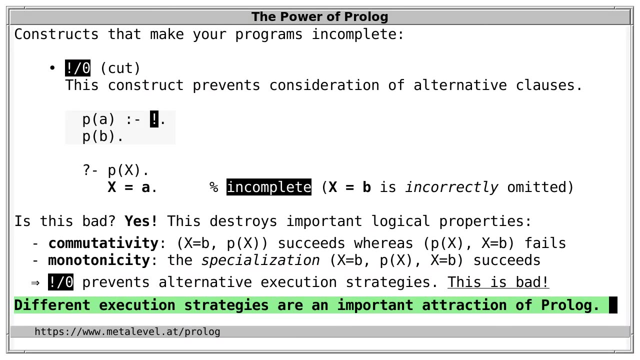 Well, as mentioned, we can only apply different execution strategies if we retain these properties And as long as there is so much Prolog code around that destroys them. we also won't hear much about alternative search strategies, But it's our goal, of course, to enable them. 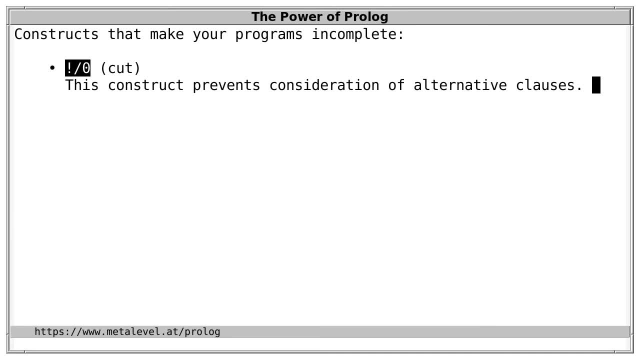 Cut prevents consideration of alternative clauses and therefore limits us to one specific search strategy. Another construct that causes incompleteness is if-then It commits to the first solution if-any of the if-part, And therefore it's only sound if the condition is ground For. 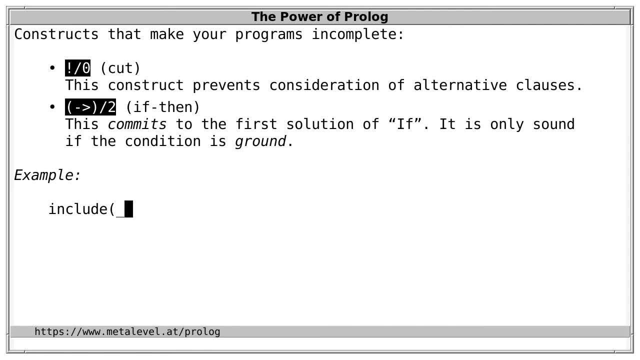 instance, let's define a meta-predicate, include, where the first argument is a partial goal, that holds for all elements of a list which are included. Then no elements are included, no matter the goal, And for lists with at least one element, it depends on whether the partial goal holds. 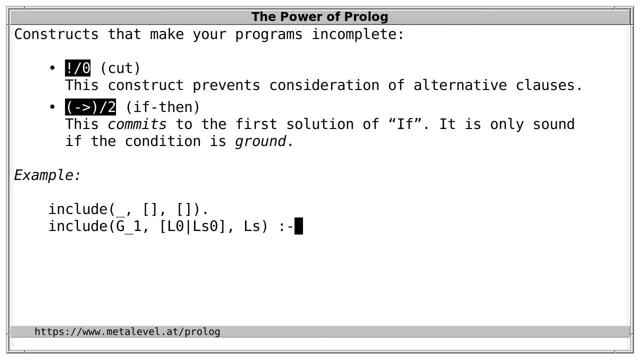 for the element. So in this case the relation holds if- and now it depends- If the partial goal holds for the first element, l0,, then the element should be included. So we relate the original list to a list ls, which contains l0 as its first element and 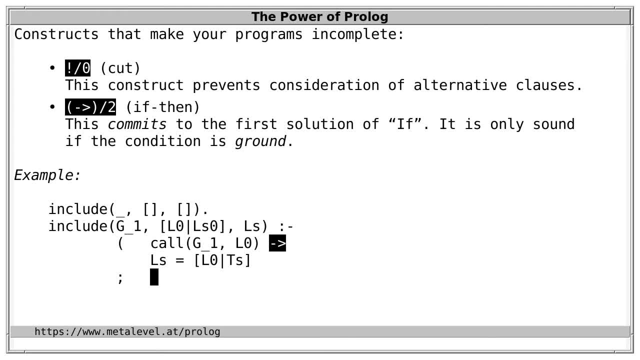 also has a tail, ts, And otherwise the element is not included. So we are making a case distinction on whether the goal holds for the first element of the list And the remainder of the list. ls0 is in this same relation with the tail of the list, with. 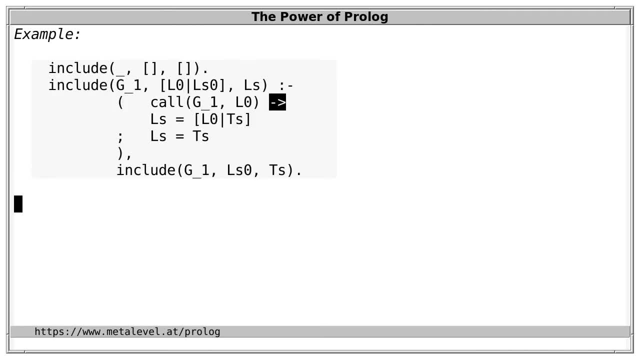 the included elements, And at first this may appear to work as intended. For example, let's ask: what are all elements greater than 3 in this list of integers And we call the list of included elements. i's Well, this is the unique solution And it's correct. So from a quick test, it appears. 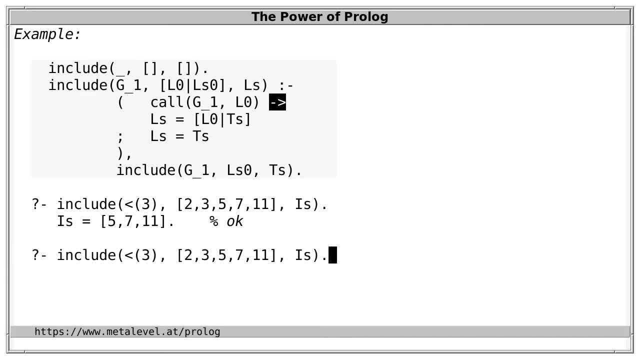 to work correctly. However, what if we take this very same query and instead of 11, we generalize this element to any term x, Because that's a unique attraction of Prolog? We can generalize our queries and ask: what about any such cases? 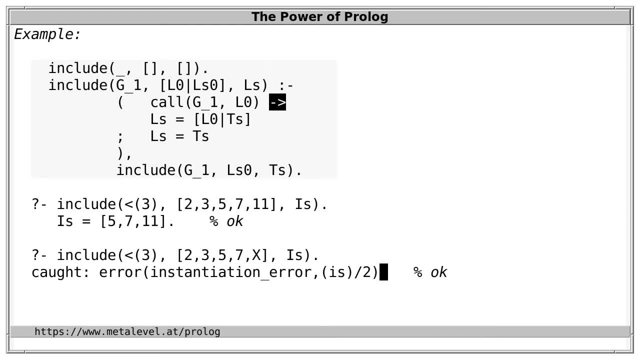 And if we do this, we get the following: We get an instantiation error, which is an OK answer. This only means that the Prolog system doesn't have enough information to make a statement one way or the other, Because there are cases where x is greater than 3 and then would be included, and also cases 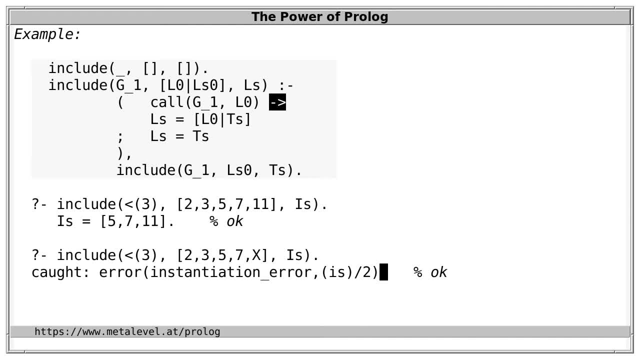 where x should not be included And the instantiation error means that, to decide this, an instantiation is expected. Now we could, of course, use a more general predicate, more general in the sense that it also works for variables. For instance, let's use the CLBZ constraint less than here. 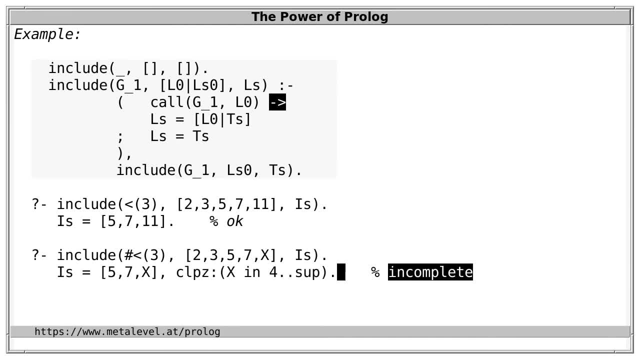 And now we get this answer, which is incomplete, Because what if x is less than 4?? Clearly, if x is less than 4, then it must not be included. However, the Prolog system has simply omitted this case and instead constrained x to be. 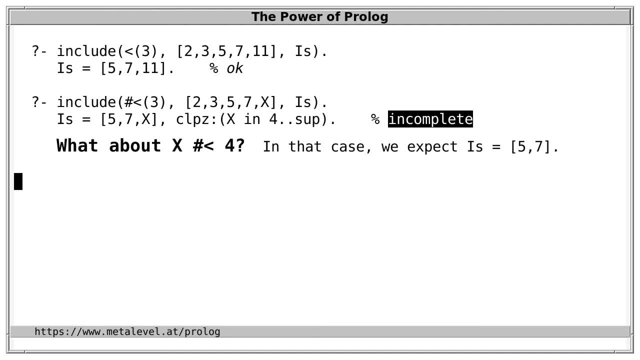 greater than 3.. And that's a huge problem because we've now lost solutions, In fact, even infinitely many. And of course there's a solution for this, because we can simply use tfilter from library rave and ask: what are the integers greater than 3 in this list? 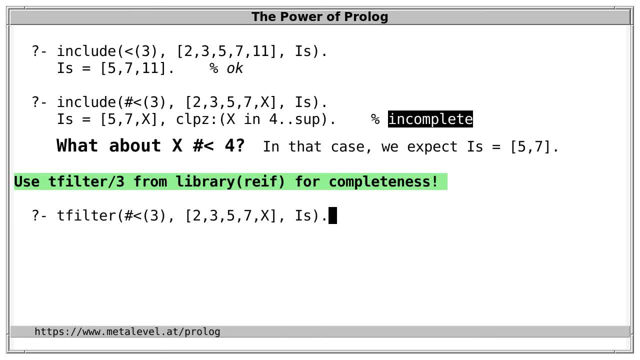 So we're now simply using the library predicate tfilter instead of our own definition of include, And now we get a disjunction. This is the first possibility: x is smaller than 4. And in that case it's not included in the list. i's. And second, x is greater than 3.. And 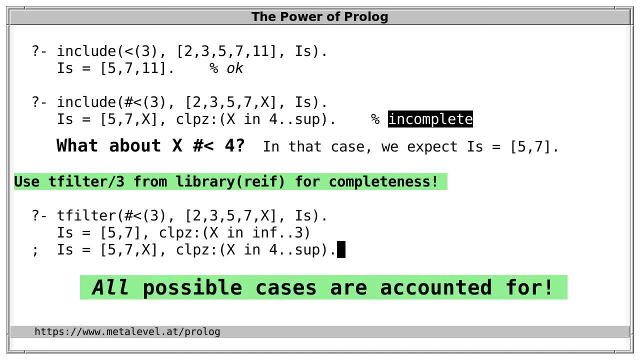 in that case it's included. So all possible cases are now accounted for And nothing is omitted. And that's of course nice. And this is what we expect from a logic program: To truthfully and completely answer what holds and what not. 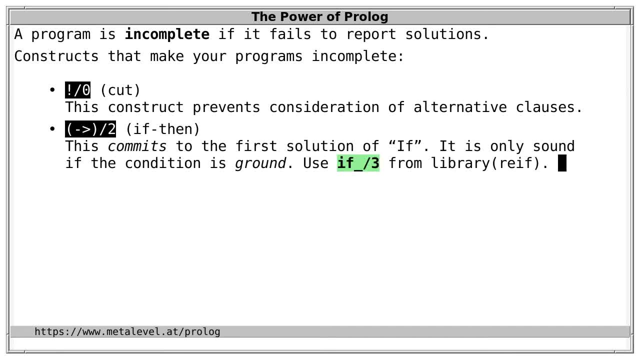 So if then is another example that violates this, And as a declarative replacement for if then, we can use if underscore from library rave. And for meta predicates such as include and exclude, which are often defined in terms of if then, and therefore also incomplete, we can use the mentioned tfilter. 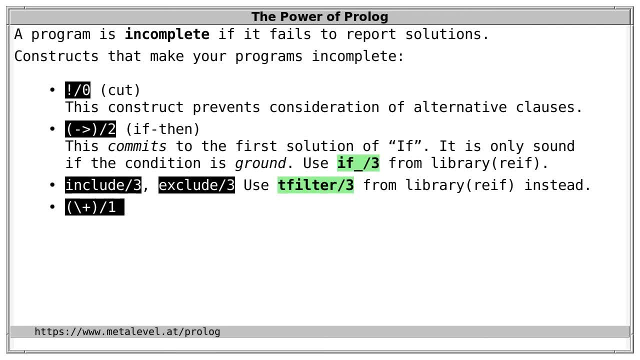 Another example that destroys completeness and therefore monotonicity is this predicate backslash plus, which can be read as not provable at this moment. So this is not negation as we know it from logic, where we'd read it as something does not hold, But it refers. 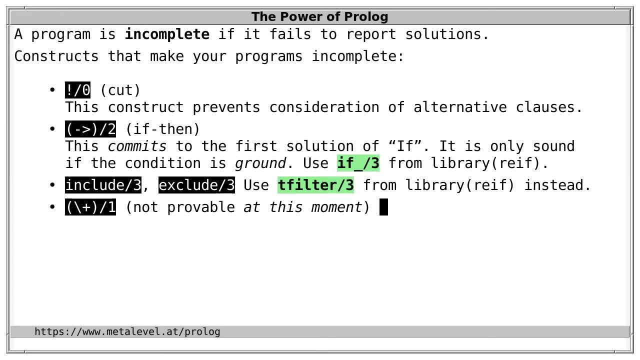 to provability at this particular point in time. So this introduces a very procedural notion into the program and again makes the meaning depend on a specific execution strategy. For instance, we can ask: is it not provable at the moment that equals of a and hello holds And we get: yes, that's not provable, However. 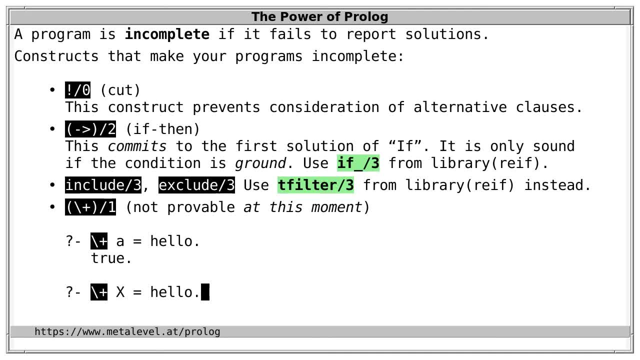 if we post a generalization of this query, namely, is it not provable that equals of x and hello holds, Then we get no, that's not not provable at this point in time. The answer is clearly because there is a solution where x is actually equal to hello, And that's. 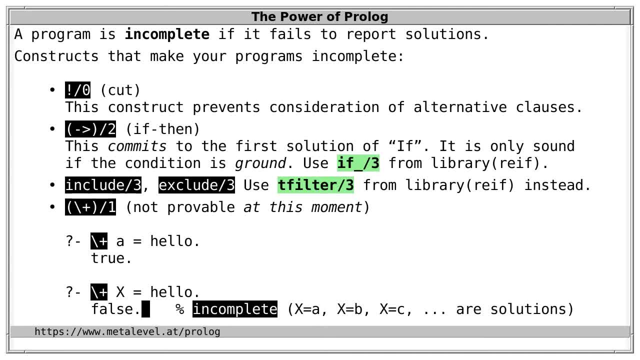 incomplete, because there are solutions such as the atoms A, B, C and of course also other terms, such as every integer and every compound term where x is really not the same as hello. And if this not provable predicate were complete, then it would have to enumerate all such cases. 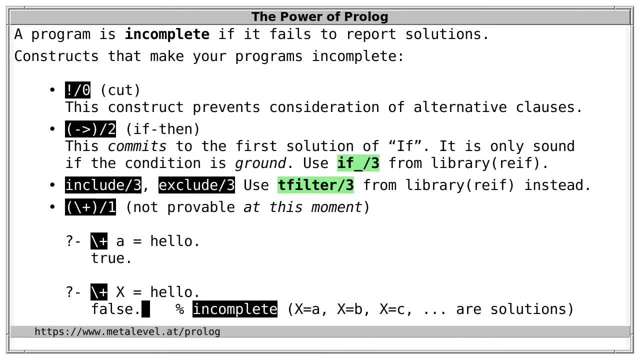 And it also depends on the execution strategy, Because if we add a suitable construct to a constraint before the goal, then it succeeds, Whereas if we added after the goal, it still fails. So not provable is incomplete, As are also other predicates such as not unifiable, 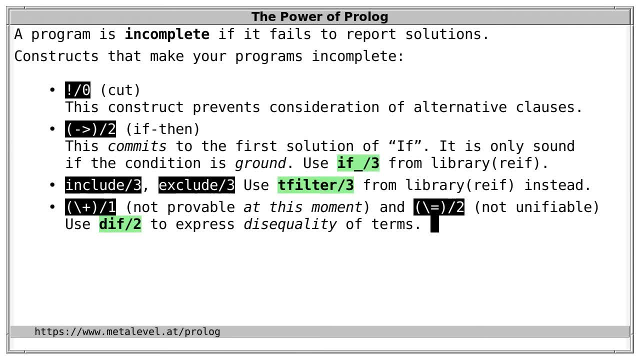 which can be expressed in terms of not provable, And also here there are good declarative alternatives, often also with a long history. For example, instead of not unifiable, simply use div to express that two terms are different, And this predicate has a very long tradition. 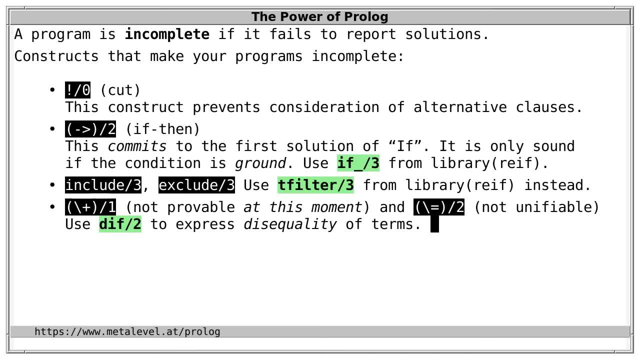 It was a already available in the very first prologue system, prologue 0.. Find all is another example. It's easy to see that find all is problematic because it can be used to express other incomplete predicates, such as not provable at this moment or checks for instantiation, For instance, if it 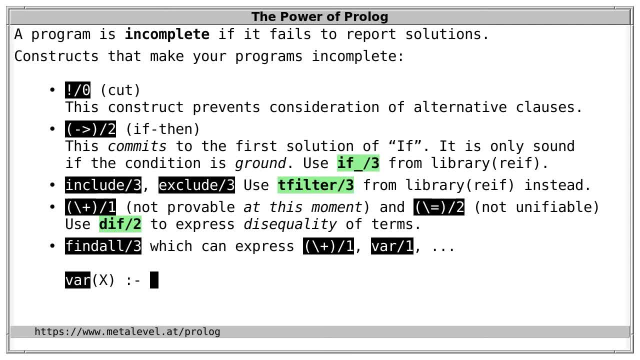 weren't already available, we could define var, which holds if the argument is a variable in terms of find. all, for example, like this: and var clearly violates commutativity and therefore prevents alternative execution strategies And also type tests such as integer, atom and so on. these are 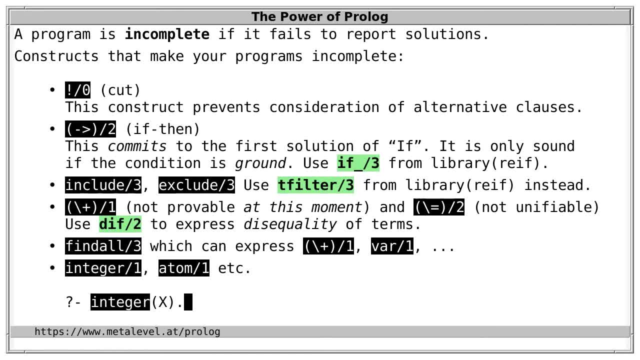 all incomplete. For instance, are there any integers? x will fail, whereas if we add a constraint it will succeed. So these type tests are clearly problematic and for correctness we use the si family of predicates instead. And incompleteness is maybe the most common mistake in prologue programs. 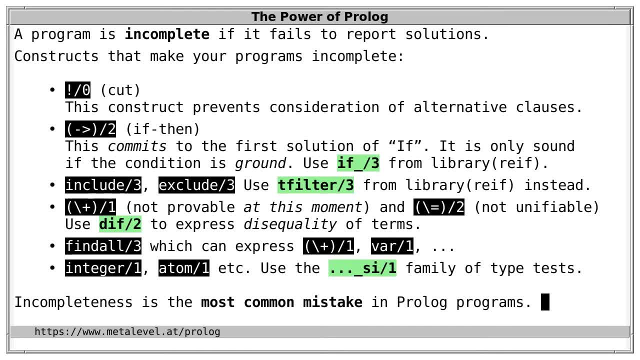 Maybe because people don't consider it as a problem, or also because they are confused about the direction of consequences. Because if we avoid such predicates, then we can reason very logically about prologue code and also run it with different execution strategies. So it's not that prologue can't be run with alternative execution strategies. 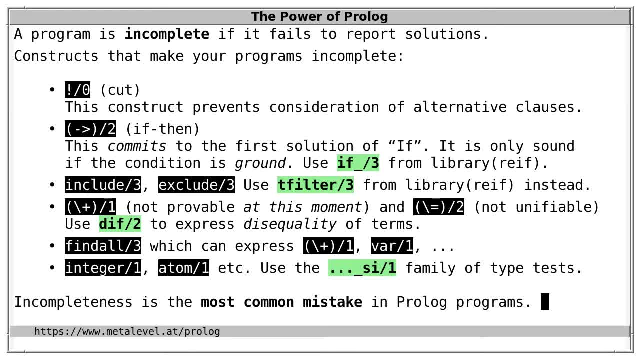 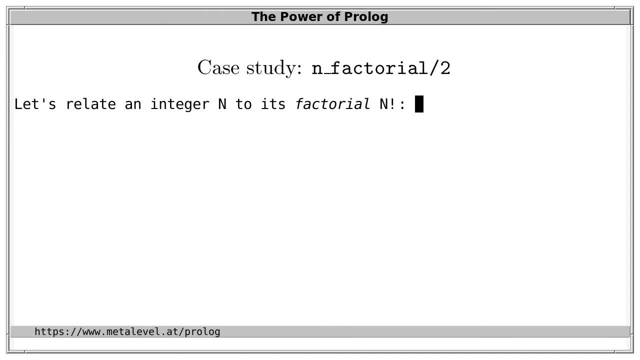 and therefore we can use these predicates Rather, the direction of consequence is: if we are using these predicates, then we can't apply alternative execution strategies. So let's consider an example. Let's relate an integer n to its factorial, So the relation n factorial holds, for if the integer is zero, then its 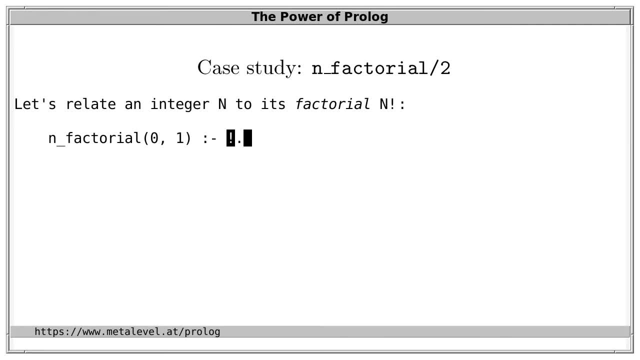 factorial is one, So in that case we don't have to consider anything else. right, And indeed we can find such code in actual practice, And we already know now that the result will be an incomplete program, But still, let's think about it. What else do we know about this relation? Well, what about n? 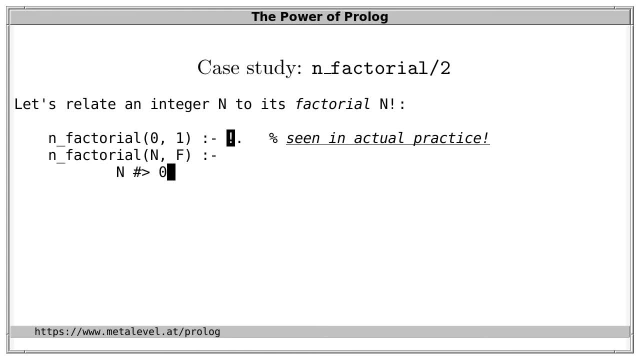 in general And its factorial f, And we've already covered the case- n equals zero. So lets now define the relation for n greater than zero. Well, in that case, if n1 is n minus 1 and the factorial of n1 is f1. 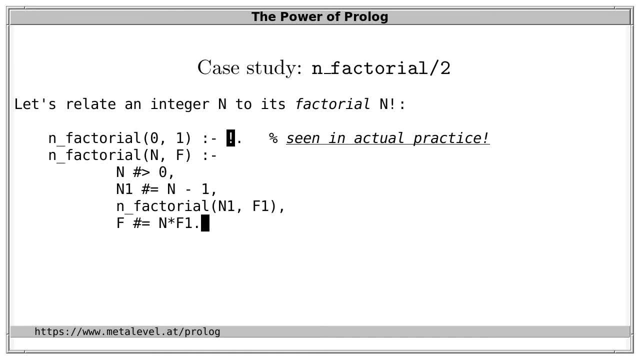 then the factorial f of n is n times f1, right, And that's it. And we can use this predicate to compute the factorial of an integer. So this mode of usage or this direction, where the first argument is instantiated, works as intended. 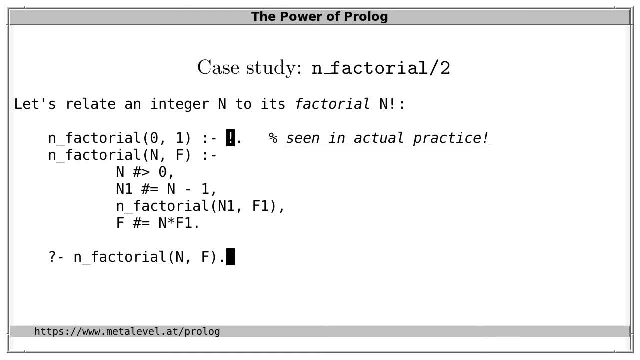 However, if we generalize this argument and ask which solutions are there in general, then we get only one solution. So the predicate is incomplete because we've used exclamation mark, And other modes also have this problem. For instance, if we instead of f ask for 1, here we get n is 0 as the only solution. 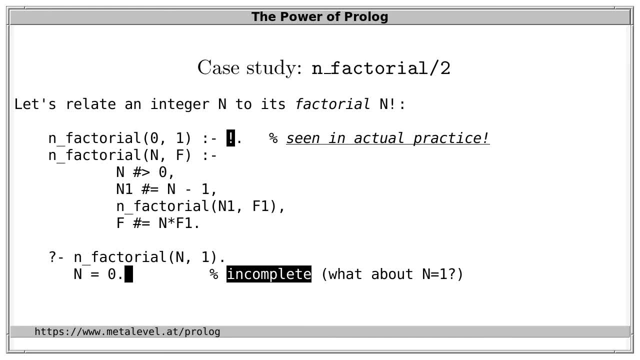 And that's incomplete too, because what about the other solution, n is 1?. So we clearly see from this example that cut forfeits the power of Prolog, Because the prime attractions of Prolog are precisely that we can generalize our programs and queries. 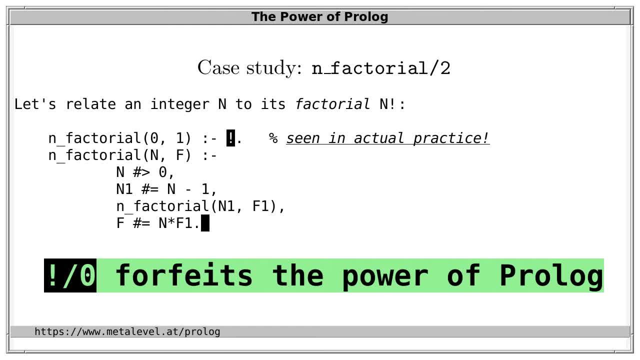 and reason about them in different ways and run them with different execution strategies, And none of this works if we destroy logical properties such as completeness and monotonicity And if we cater to only one particular execution strategy by using predicates that only have a procedural reading. 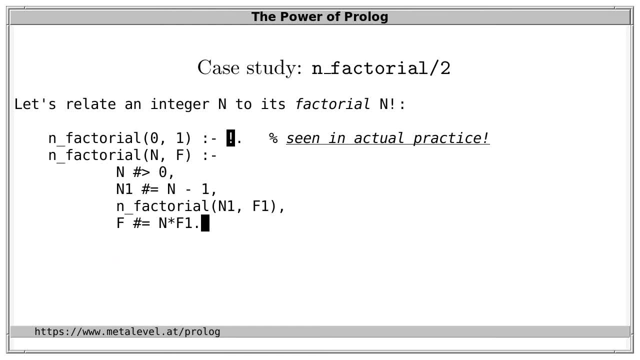 instead of a declarative one, And we solve this problem by simply removing the cut. And if we now post the same query as before, we get the same solution as before, And Prolog also tells us that this is the only solution. So the choice point was entirely. 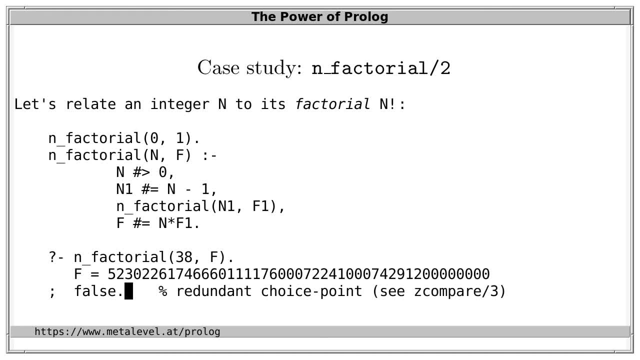 In fact redundant here And if we want we can use z compare to prevent the redundant choice point. But this is only a matter of performance and doesn't change the meaning of the program in any way, Namely the set of solutions it describes. 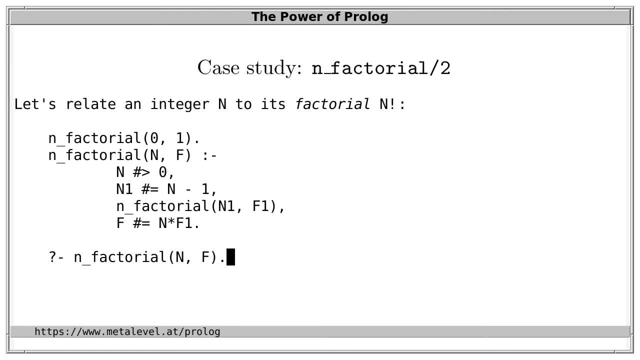 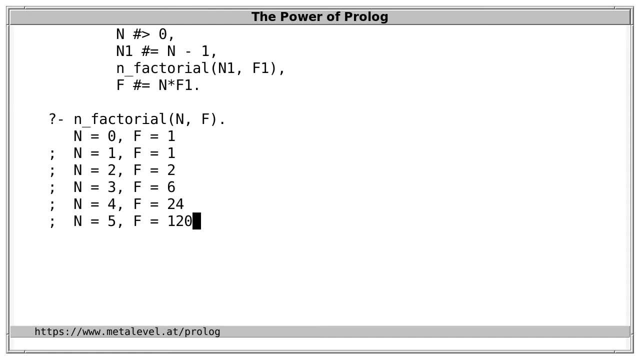 And further. if we again generalize the query and ask: which solutions are there for any n and f, then we get this solution as before and also others. So now the predicate enumerates all solutions. So that's nice. And if we focus on just 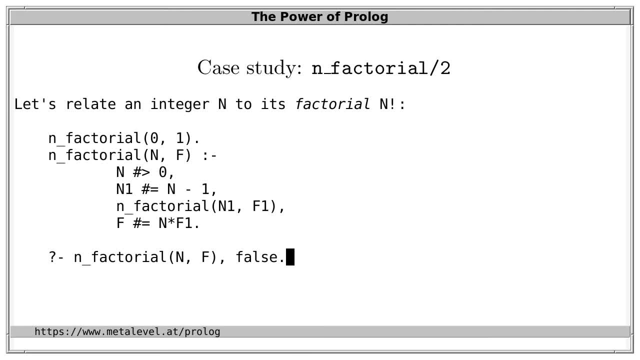 Just termination by adding false here. So we don't expect any solutions now, because of course this can never succeed, But focus only on whether the predicate terminates. Then we see that the query doesn't terminate as expected Because there are infinitely many integers for which the relation holds or ought to hold. 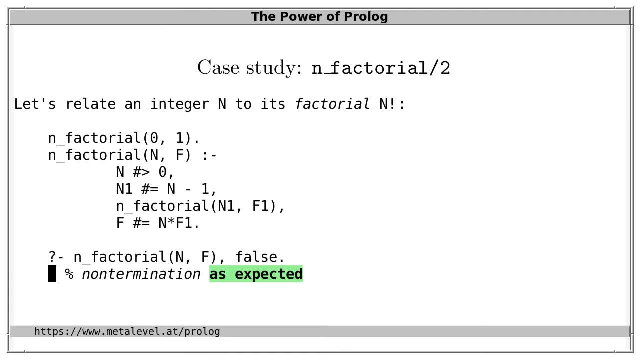 And if it's complete, then it must not terminate. So it would be a programming mistake if we could observe termination here. Now. what about Our other example from before, where instead of f we ask for all integers whose factorial is 1.. 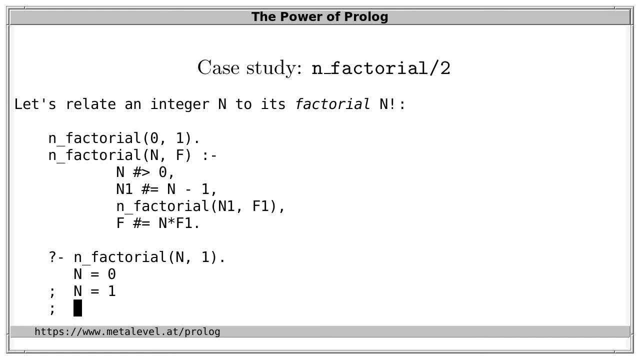 Now we get 0, as before, and now also 1.. And then it doesn't terminate, Which is okay. It's not wrong to not terminate. What is wrong, though, is to explicitly say there are no or no more solutions, when in fact, there are solutions. 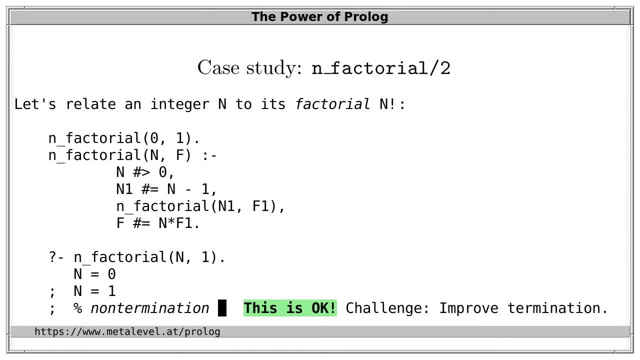 But still it would of course be preferable if this query also did terminate, Because we know that there are no solutions, But still it would of course be preferable if this query also did terminate, And so there are no other solutions. 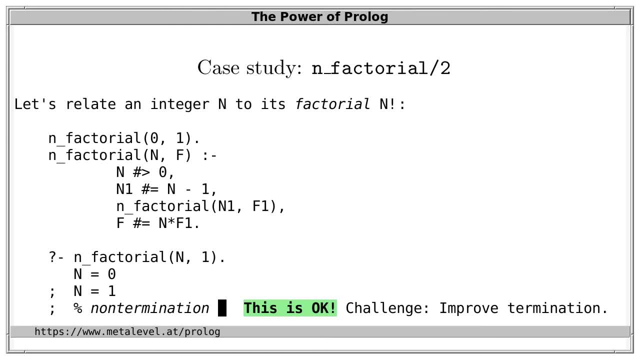 It's just that, with the default execution strategy, Prolog does not derive this, And we can help Prolog to derive this First. if you think about it, then f can only be greater than 0, right, So we can add this as an additional constraint. 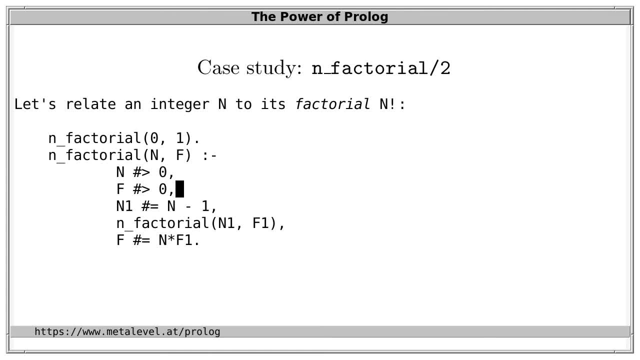 And we know that CLBZ constraints always terminate And therefore adding such a constraint can at most improve termination, never by itself cause non-termination And therefore adding such a constraint can at most improve termination, never by itself cause non-termination. 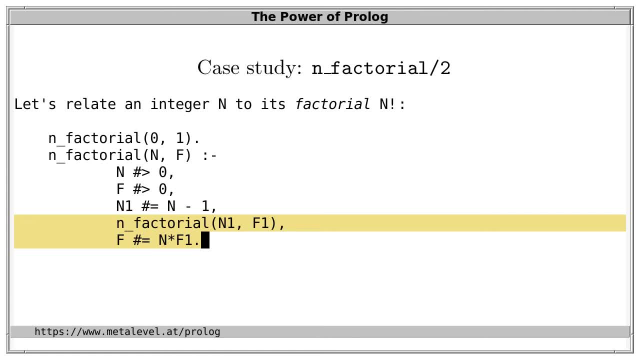 And another thing we can do to cater to the procedural semantics of the default execution strategy is to reorder goals, And we can do this because we are using general predicates. So because we are using predicates that can be read declaratively, such as CLBZ constraints, we can reorder goals. 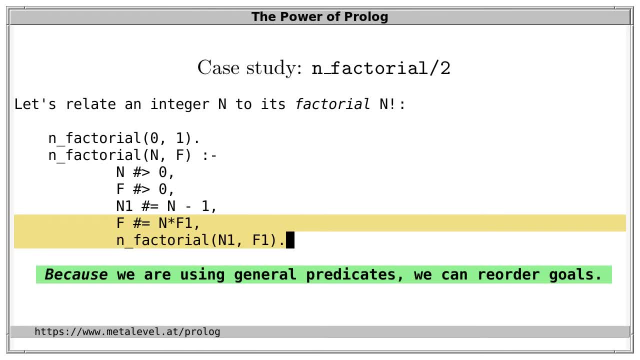 For instance, we can simply exchange the last two goals so that the CLBZ constraint, which we know terminates, is placed before the recursive call. And with this definition, when we post our query from before and only consider its termination properties, then we see it now terminates. 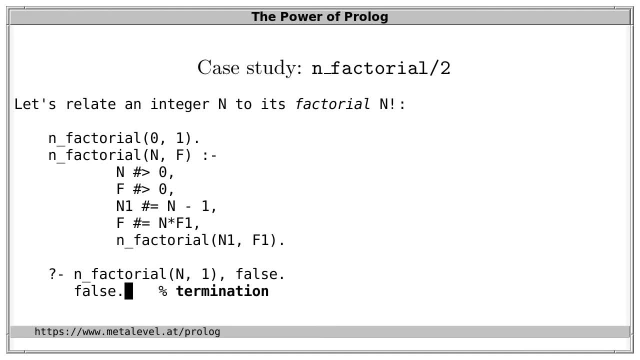 So with these simple changes, we've improved the termination behavior of our program. Of course, termination is not all that matters, And our changes may also have other effects. For example, they may have made the program slower in some cases. But even apart from performance, a huge problem still remains. 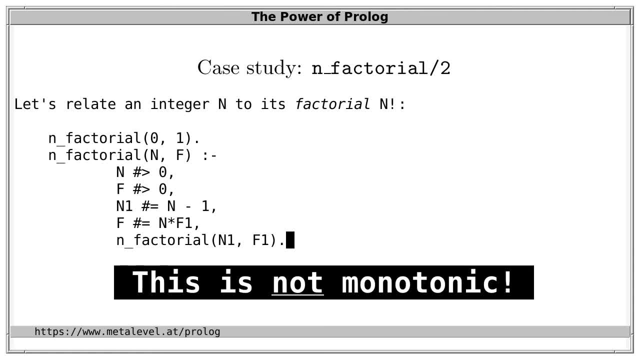 And it exists in all versions of the program we've seen so far. Namely, this predicate is not monotonic And therefore it's not amenable to different execution strategies, Because it will report wrong answers, For instance, if we ask: is there an integer n? 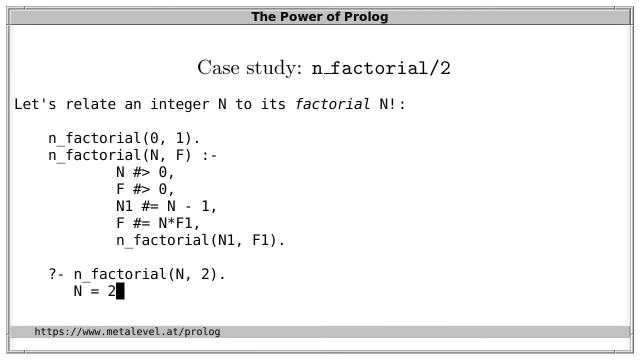 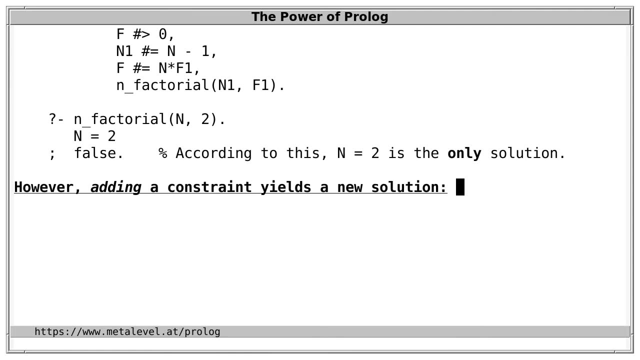 Such that the factorial of n is 2,. then the program tells us: yes, n is 2, is a solution and no other solutions exist. So, according to this answer, n is 2 is the only solution. However, adding a constraint yields a new solution. 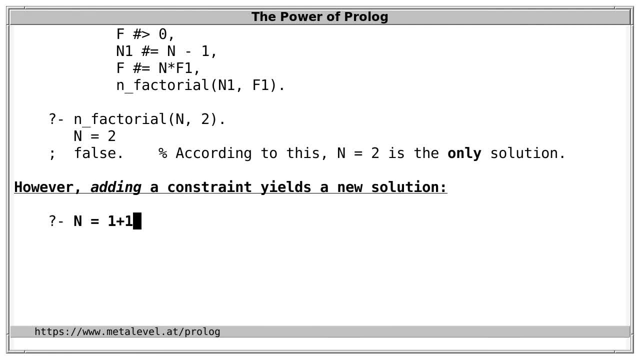 Because if we state that n is the compound term- 1 plus 1, so not an integer but a compound term- and then ask: is it the case that n factorial of n and 2 hold? And then ask: is it the case that n factorial of n and 2 hold? 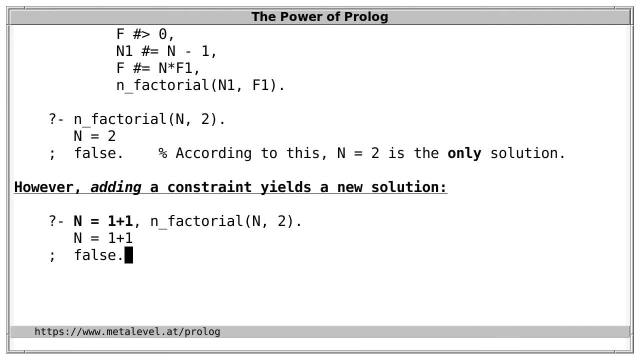 We get: yes, this holds, And n is 1 plus 1 is the only solution. So that's a huge problem, because it means that we can't rely on what the program tells us. Who knows what other solutions there are too. 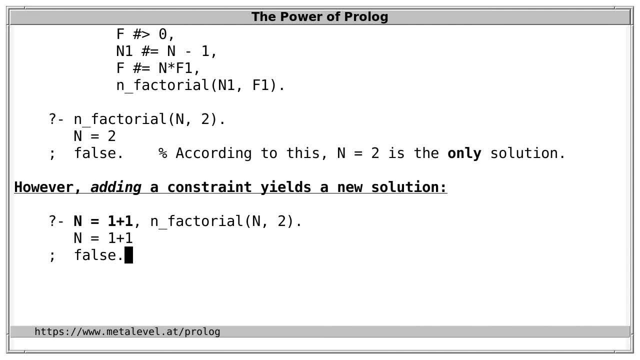 So what we want from the program is, of course, the truth about the situation. If the program tells us there are no other solutions, then there shouldn't be any other solutions, Especially not if we add additional constraints, Which should only be able to remove solutions, certainly not add them. 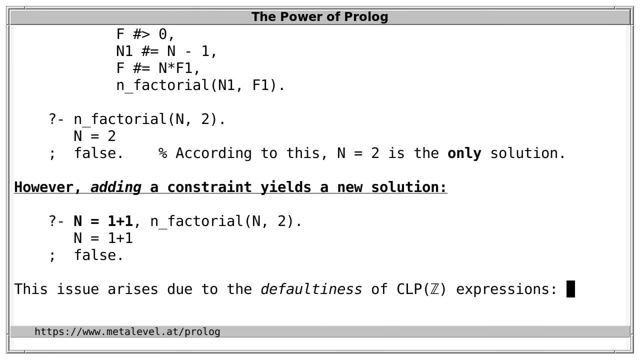 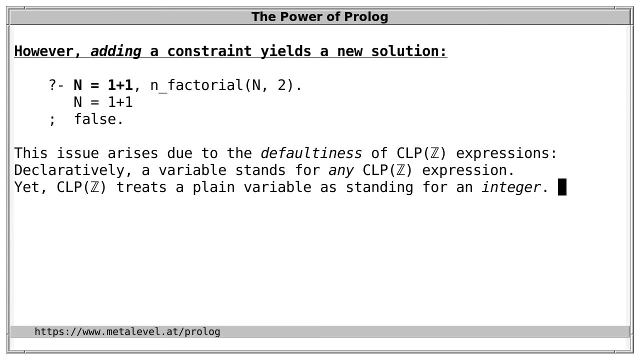 And this issue arises here due to the defaultiness of CLBZ expressions, Because declaratively a variable in an arithmetic constraint stands for any CLBZ expression, not just concrete integers. Yet CLBZ implicitly treats a plain variable as standing only for an integer, never a compound expression. 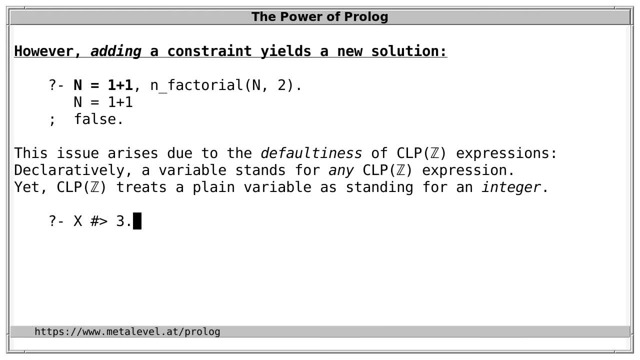 For instance, if we ask for which x Does x greater than 3 hold, Then CLBZ tells us it holds for integers, and only for integers, between 4 and positive infinity. But we know, of course, that there are other solutions for x too. 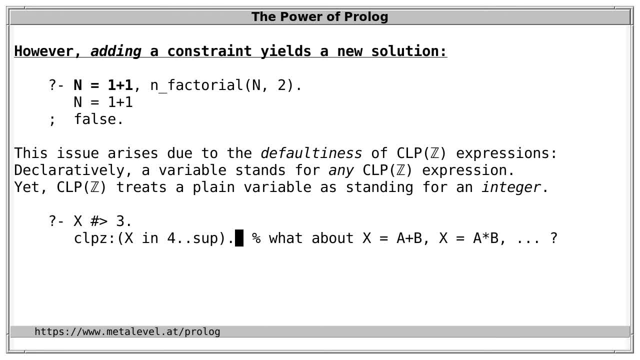 Namely compound terms such as a plus b, a times b and so on, For instance. we know that the compound term 2 plus 2 is also a solution, And to solve such problems we use the wrapper number sign. 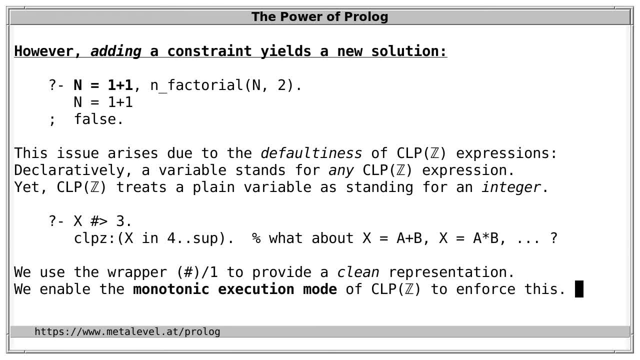 To provide a clean representation And we also enable the monotonic execution mode of CLBZ to enforce this. So, for instance, in Scriapolog we assert the fact CLBZ monotonic to enable this mode, For example by using the standard predicate assertZ, which asserts this fact. 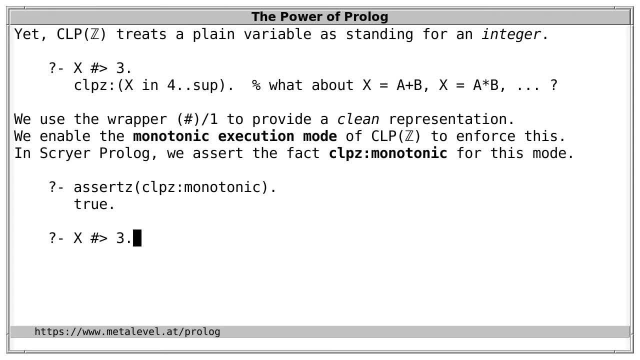 And in the monotonic execution mode, if we post is there any x for which x greater than 3 holds, We get an instantiation error, which is perfectly okay. It simply means that the argument is insufficiently insufficiency, So we instantiate it to give a definitive answer. 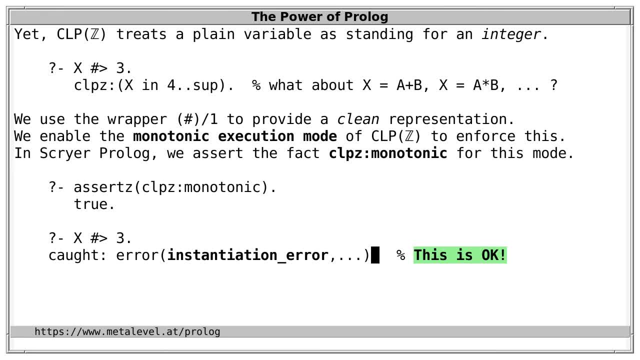 And also in this case terminate, Because clearly for completeness Scriapolog would have to enumerate all terms, also compound expressions, for which this predicate holds. So in the monotonic execution mode we must use the wrapper. So we write number: sign of x greater than 3.. 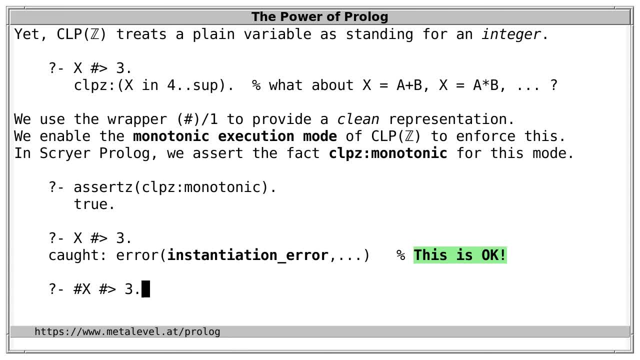 So we make clear here that we're talking about concrete integers, not about compound expressions. And then see, CLBZ gives a complete answer. This holds if x is an integer greater than 3. And x can really only be an integer, because the predicate in only holds for integers. 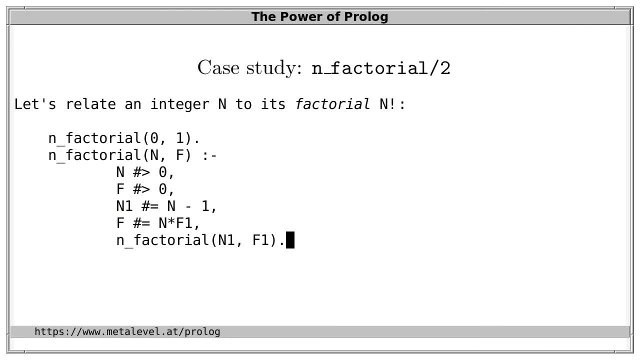 not for compound expressions. So we now apply this to our program. We simply use number sign to indicate variables that we mean to stand for concrete integers, not compound expressions. So for instance, by the task description we mean this n here to stand for a concrete integer. 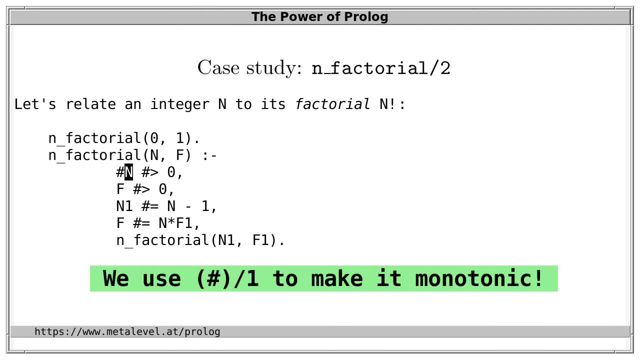 And so we add the number sign, Number sign wrapper. That's really all there is to it. It's a straightforward and small syntactic change to the program. Also, this f- here We mean it to denote the factorial, which is an integer. 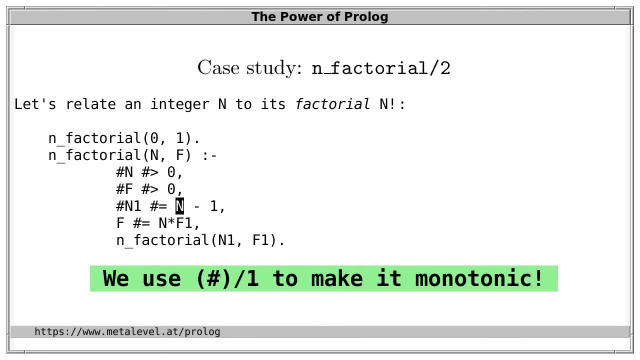 And this n1 as well, And here n again. We've already indicated that it must be an integer, and it's okay to do it again here. Number sign of n And also again number sign of f, Then n again and also f1. 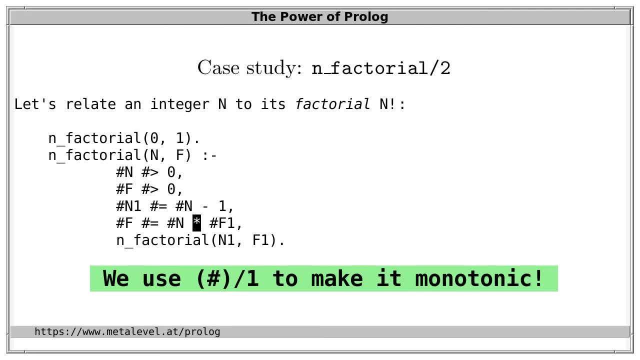 And we add a space to make this syntactically valid And for symmetry also. And that's all. So now, with these added number sign wrappers, our program is monotonic. And if we ask, for example, for which integers n is the factorial 2,? 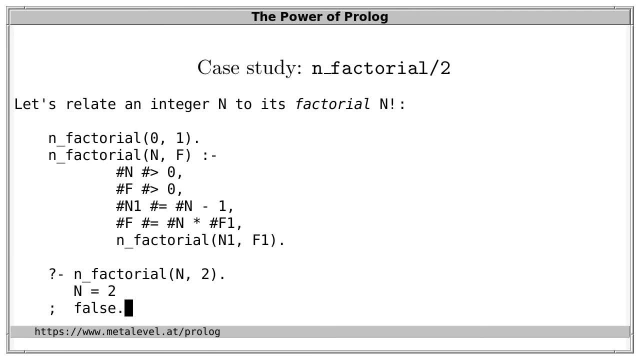 we get the solution: n is 2, and it terminates all exactly as before And in contrast to what we had before. if we add the constraint, n is the compound term 1 plus 1, then we get a type error, Because a compound term is not an integer. 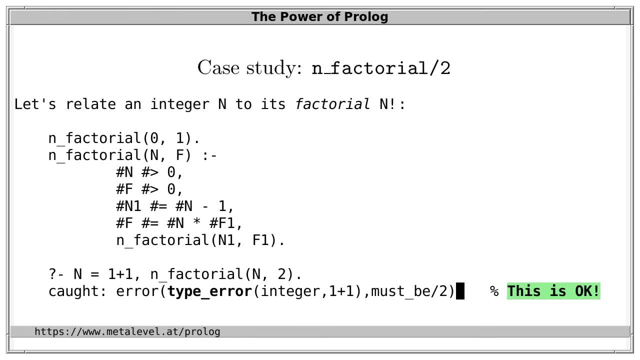 And this is okay, because we meant the predicate to hold only for integers, Not for compound expressions, And a type error, in contrast to an instantiation error, can be replaced by silent failure. So read declaratively: this simply means that the predicate does not hold for this compound term. 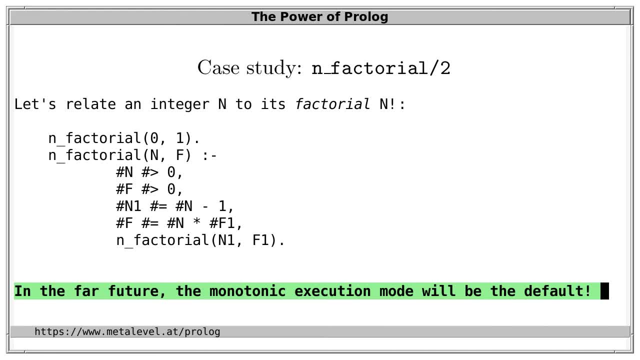 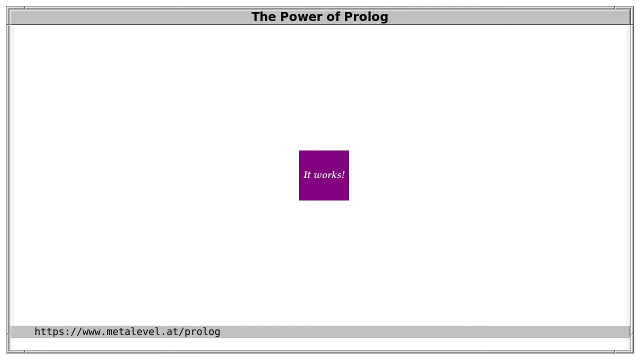 And our goal is, of course, to make the monotonic execution mode the default. Of course this will take a very long time, And one may say: is this really so important? I mean, after all, for the simple things we meant to do with the program, it worked correctly. 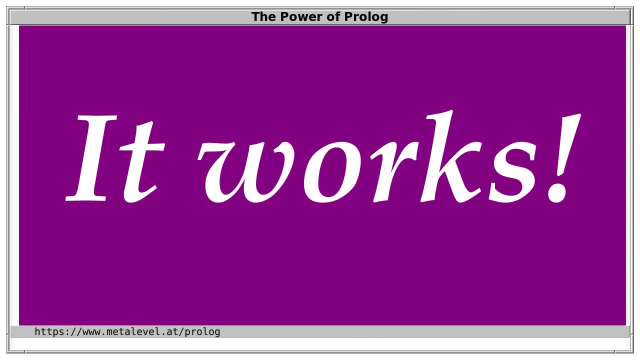 And indeed that's true. However, what about all the other things we could have done with the program and which didn't work? We probably didn't even think of them yet there are so many things we can now do with the program. 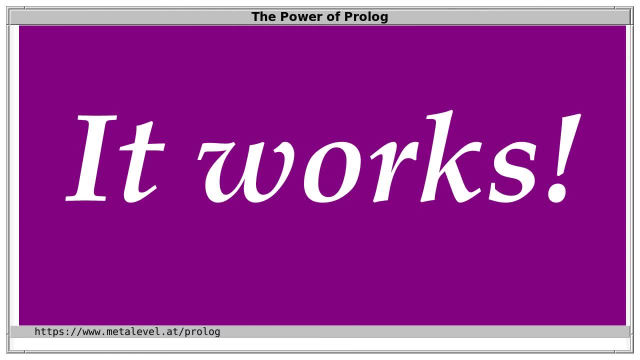 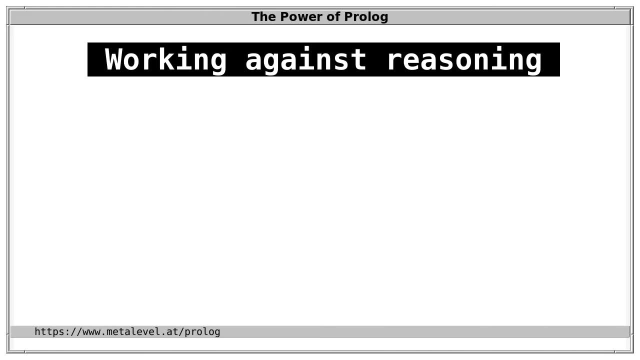 in addition to the simple things that already worked in a sense. And speaking of working and to generalize from this specific mistake, namely incompleteness, one could say that a very common mistake by programers is that to work against reasoning. 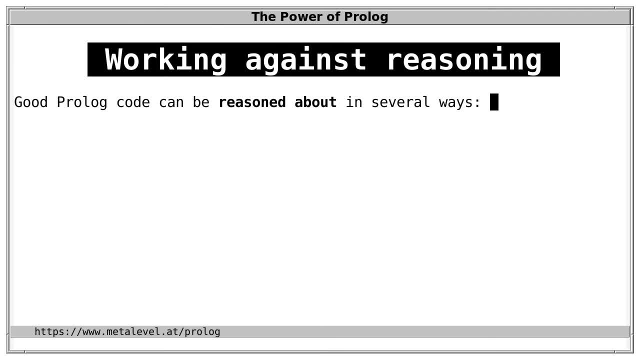 Because a decisive property of good Pollock code is that it can be reasoned about in several ways, Starting from extremely basic things such as using queries to ask the Pollock system for what holds, And also to use these queries to write test cases. 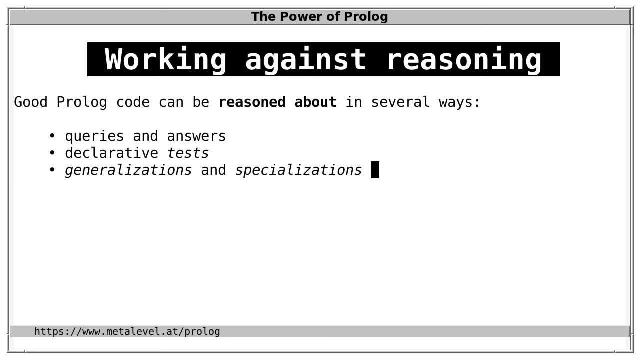 And further to generalize and specialize queries and programs, to find out more and to locate mistakes, Or to perform experiments, For example various kinds of termination analysis, For example via abstract interpretation, which can also be used for type checking and also type inference. 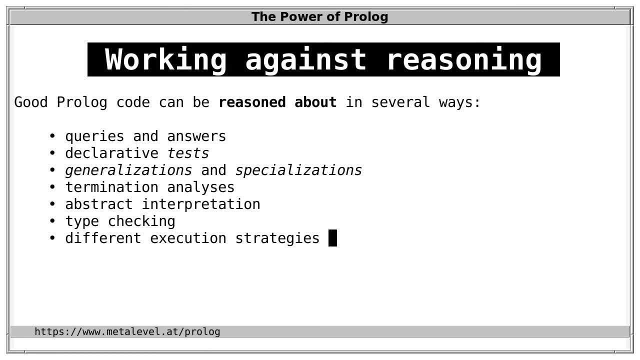 And we can also interpret the code with different execution strategies and so on. And all these examples of reasoning rely on properties that must be preserved, And the more properties we preserve, the more reasoning we can easily apply and automate. And if we break these properties, then reasoning becomes harder and harder. 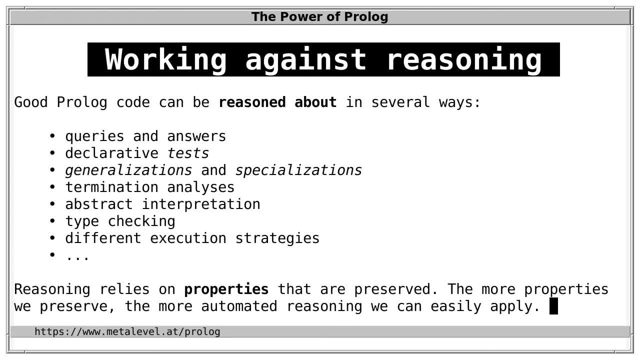 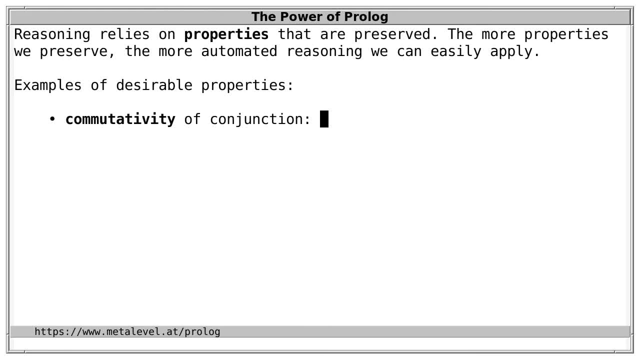 Often to such an extent that we can't really apply it at all anymore, at least not easily, And we've already seen examples of desirable properties, such as commutativity of conjunction, which means that we can rely on A and B to mean the same as B and A. 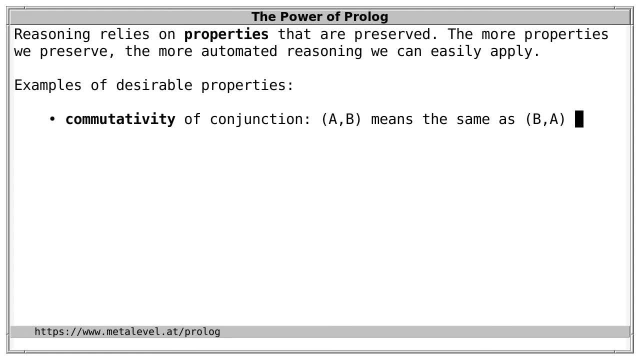 So we can exchange goals and therefore also automatically try different orders of goals to deduce logical consequences Or monotonicity, which means that adding a constraint can at most yield fewer solutions, never more solutions. Another desirable property is idempotency, which means that stating a goal G once, 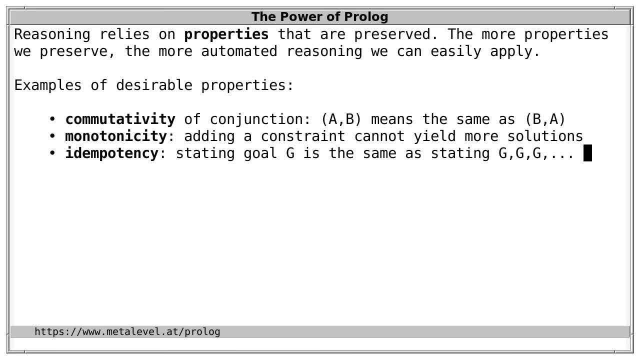 means the same as stating it several times. So with this property we can automatically eliminate duplicated or entailed goals. Another property could be called separability- Maybe there is a better name for this- but what I mean with this is that clauses and predicates 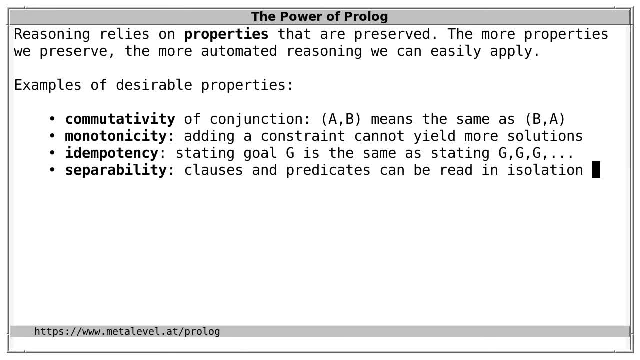 can be read and reasoned about in isolation. For example, cut violates this because it introduces dependencies between clauses of a predicate And another property, for which I also don't have a better name at the moment, could be called accessibility. I mean that all relevant things are amenable to reasoning. 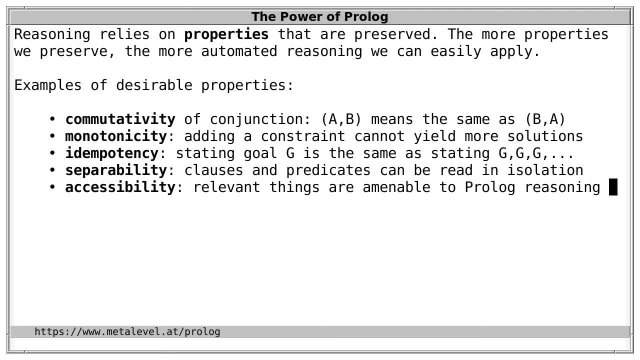 So how do we ensure these properties? Well, for commutativity and monotonicity, we already know that we must avoid certain predicates that violate these properties, such as exclamation mark if-then not-provable-at-this-point-in-time. 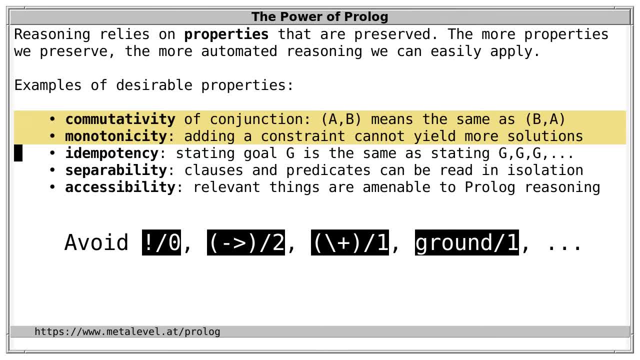 non-monotonic type tests such as integer atom and so on, and also metalogical predicates such as var ground and so on. And also we must enable the monotonic execution mode of CLBZ so that integer constraints are also monotonic. 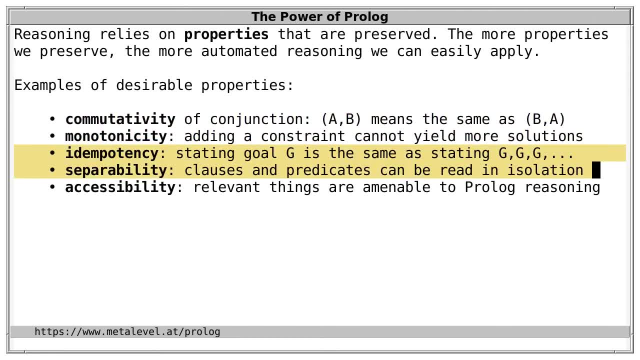 Then, to guarantee idempotency and separability, we must avoid certain additional predicates, most notably assert and retract, which are predicates that change the clause database at runtime, And the problem with this is that the clause database is global and implicit. 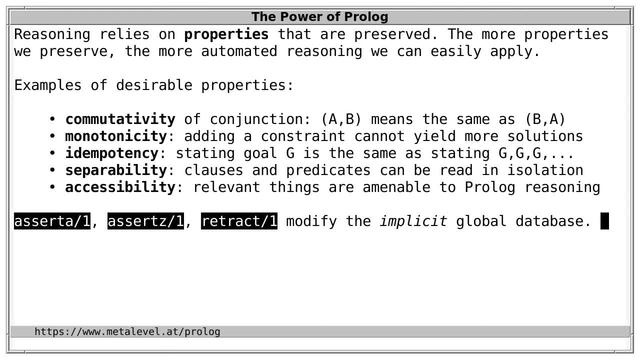 So this violates separability, because other predicates may be affected by this, And in addition, asserting a clause twice also adds it multiple times to the database, So it violates idempotency too, And also such changes to the clause database are also not undone on backtracking. 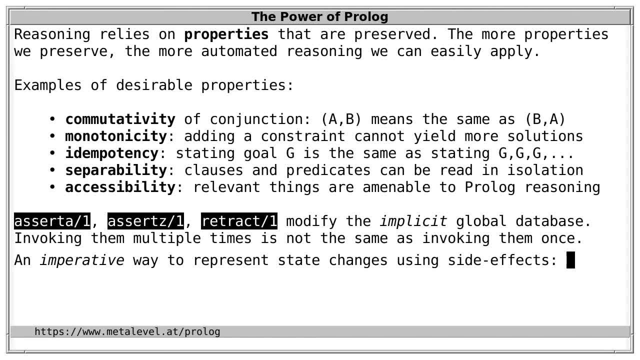 And therefore these predicates are sometimes used to imperatively express state changes. that is where we destructively modify a state to express changes and therefore can no longer truly reason about the change, And we call such a change a side effect of the predicate. 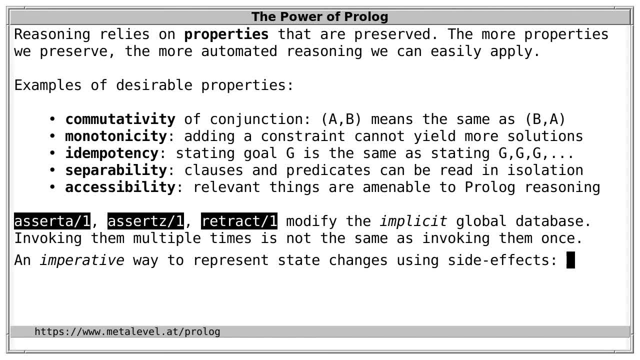 because it's something that occurs outside the declarative meaning, Because declaratively asserting a fact simply succeeds. But it does have an effect beyond this because it leaves an additional clause in the database that will affect other predicates from then on. For instance, we may have a predicate that reflects the information. 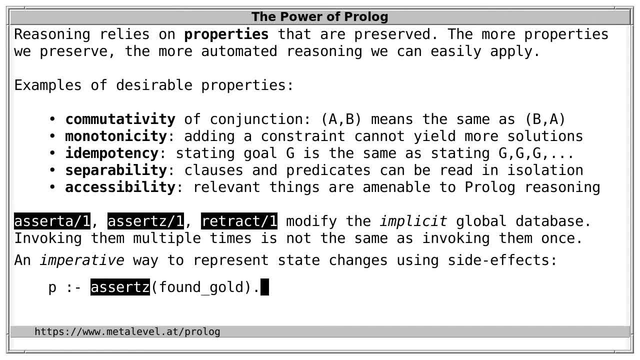 that an agent has found gold, say, by asserting the fact in the global database, which is a non-local effect, because we are adding a new fact and this may also affect other predicates from now on. So we've now created a runtime dependency between predicates. 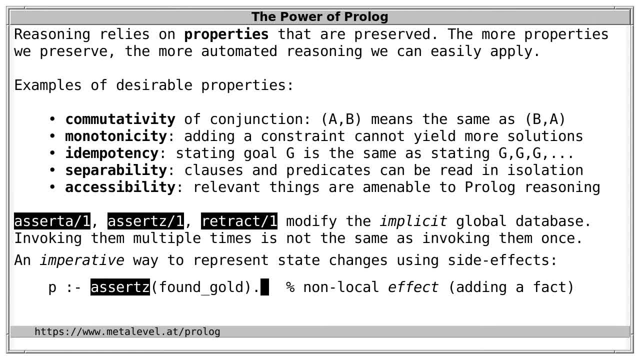 because the fact found gold depends on whether P was executed or not. And when we reason about this fact in other predicates, then their meaning implicitly depends on the predicate P, even though P doesn't appear in the clause body. So if we destructively change the clause database, 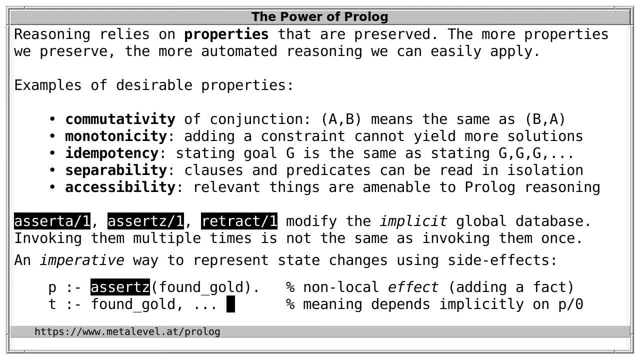 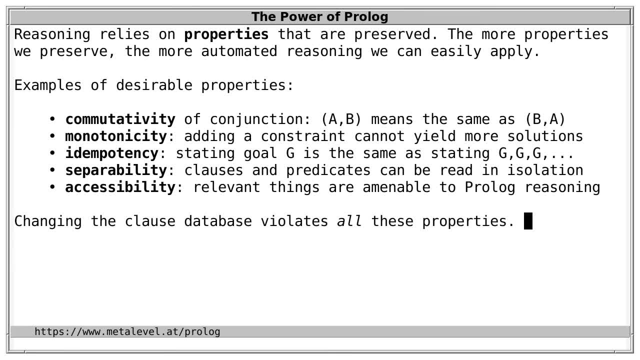 then we can no longer reason about predicates in isolation, And this significantly complicates testing, for example. So changing the clause database at runtime violates all these properties, and we therefore always try to avoid it. Instead, we describe changes declaratively. 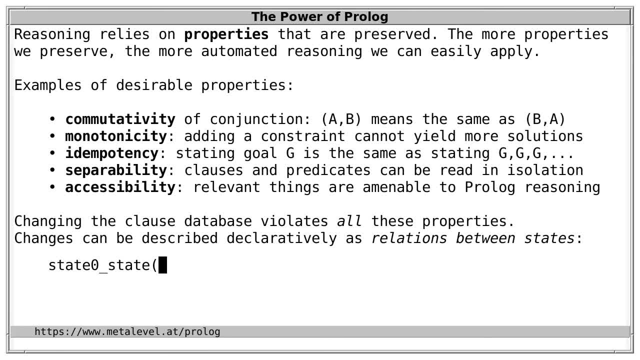 as relations between states. For instance, in our example agent we could have a predicate state 0 state where we relate the current state- state 0, to the next state. if something holds And depending on the situation, one of the next states could, for example, be that. 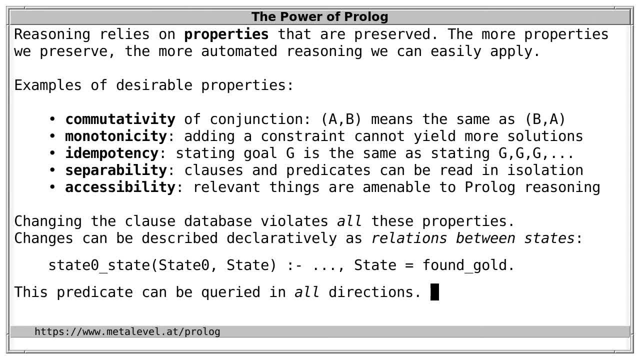 the agent has found gold, And now we have the advantage that we can query this predicate in all directions. We can, for example, ask what are possible states in which we can find gold, Or, for example, which state transitions are possible at all. 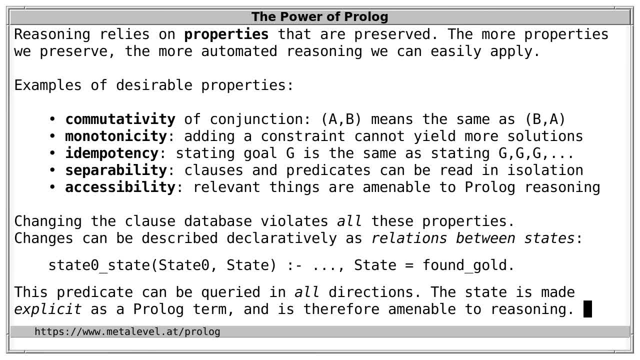 And we can now do this because the states are now available explicitly as prologue terms and can now be queried and reasoned about. So this is what I mean with accessibility: We have access to the things we are interested in. They are available as prologue terms. 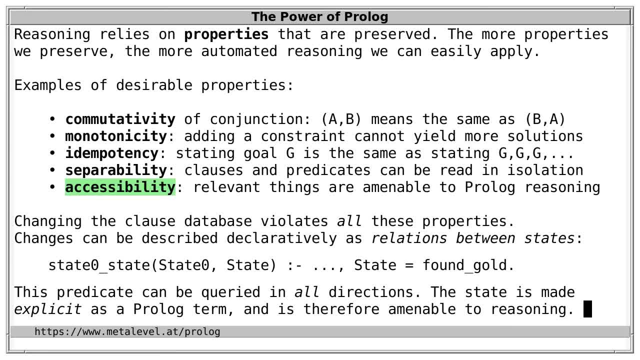 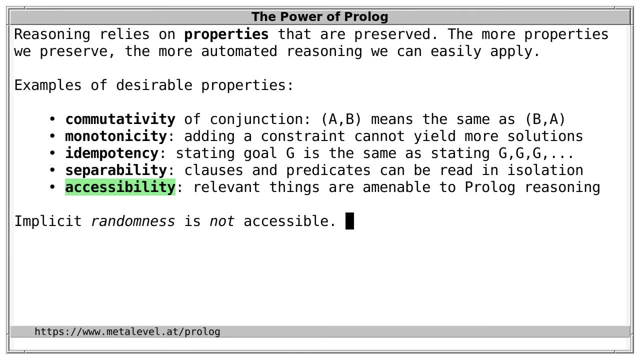 Whereas, in contrast, if state changes are expressed as destructive modifications to the global clause database, then we cannot reason about them in this way. And, as another example of this, implicit randomness is not accessible. So if we invoke a predicate to generate, for example, 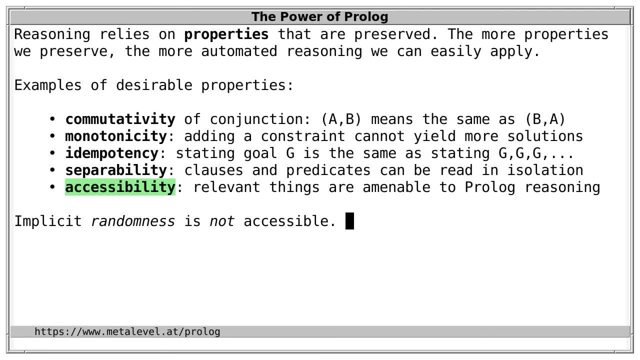 a random integer and there's an implicit state that determines which integer is next, then it means that there's something in our program that escapes prologue-based reasoning, And the program is therefore no longer entirely logical, but depends on something beside the declarations. 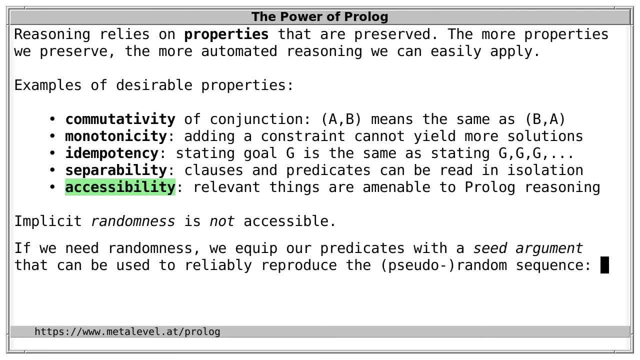 And that's what we call collaborative semantics. And a solution to this is to introduce an explicit seed argument. Because if the random seed is available explicitly as a prologue term, then we can use it to reliably reproduce the outcome of our program. For instance, if we want to express a random 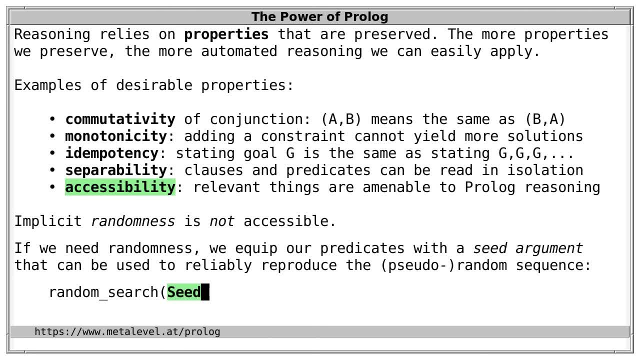 or pseudo-random search in prologue. then we would do this with a seed argument And the seed can be used to initialize the random number generator. And of course, there may also be other arguments, such as a list of variables that must be labeled and so on. 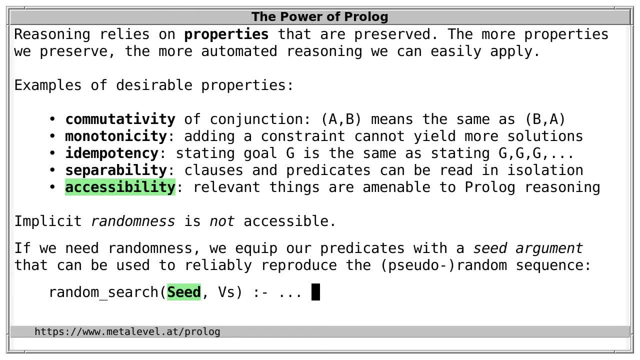 The point is that if we specify the same seed, then we always get the same outcome And therefore we can reason about the program and analyze, for example, why a test case failed and so on. So again, we've made the state accessible as a prologue term. 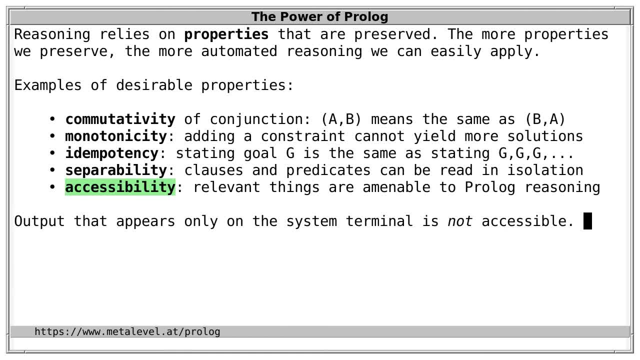 And as yet another example of this, consider output that only appears on the system terminal. Again, that's a side effect of predicates that write output, because declaratively they simply succeed, But as an effect they change what you see on the terminal. 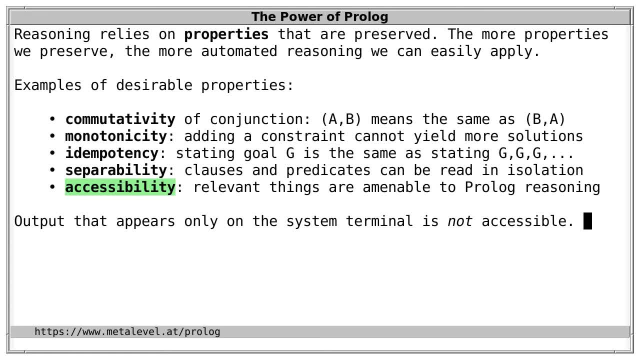 And these are destructive changes because they are not undone on backtracking. So a predicate may also write output and then fail, and yet the effect remains. And especially from beginners, we often see Apollo predicates such as main, which is true if s is a solution to a task. 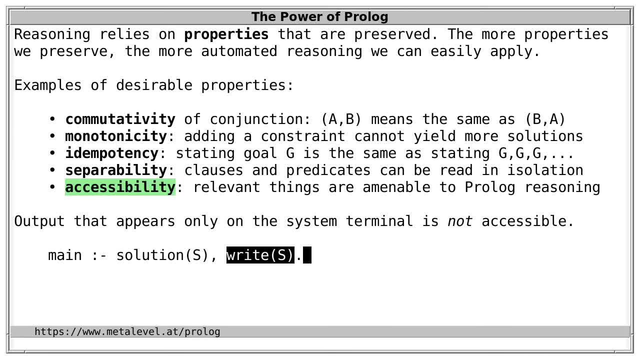 and which then writes s on the terminal. And the issue here is: how do we test this predicate? Because the output only appears on the terminal and we can't, at least not easily reason about the output with prologue. Of course we could write a separate program for this. 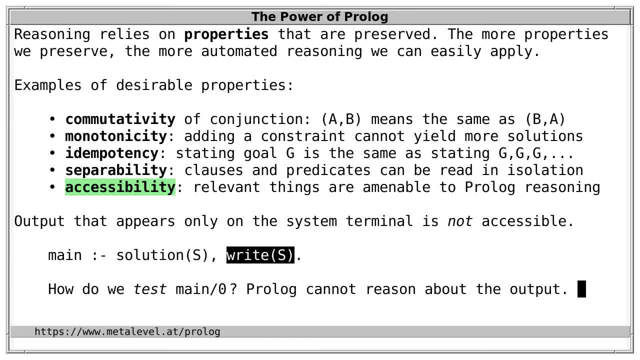 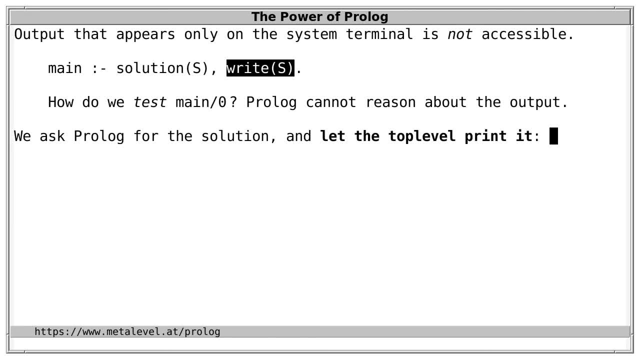 but, in all honesty, who really does this? And therefore you'll most likely not write tests for the output. So what we should have done here is to simply ask for the solution and let the top level print it. Simply post a query. 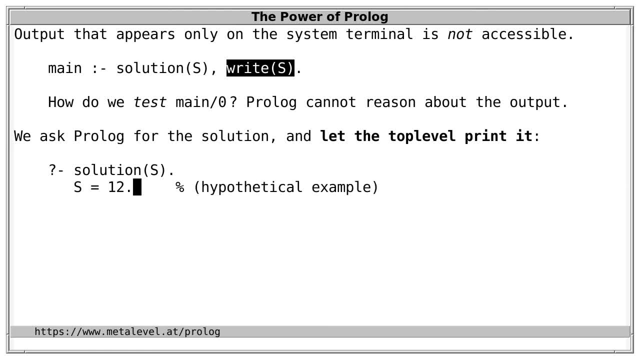 and the top level will automatically show the answer. as in this hypothetical example, And for more complex output, we can use the dcg non-terminal format underscore to describe the output as a string, that is, a list of characters. For instance, we could introduce a non-terminal formatted solution. 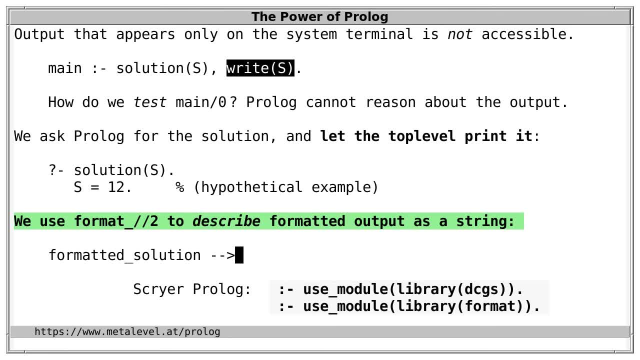 using a dcg to describe the list. So for example, in scry Apollo we load the dcg's library and format underscore is in library format And here we state for example: if s is a solution, then the output we want to describe. 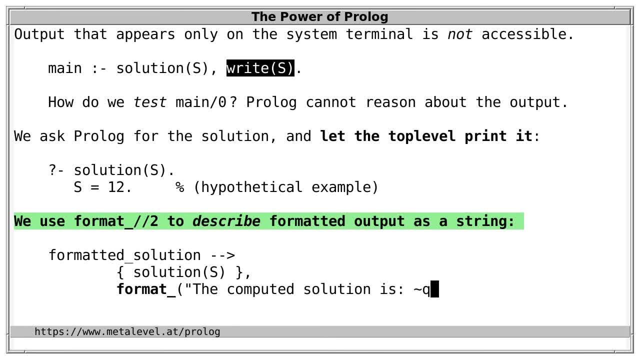 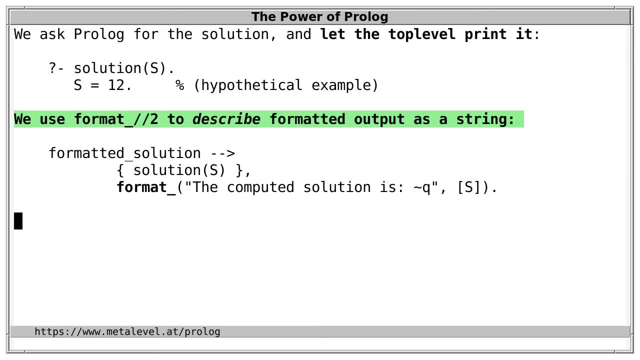 is a list of characters that also contains the quoted solution s, And we call such a specification a format string, because it specifies the format of the output. And the second argument is a list with terms that are referred to in the format string, And the advantage is clear. 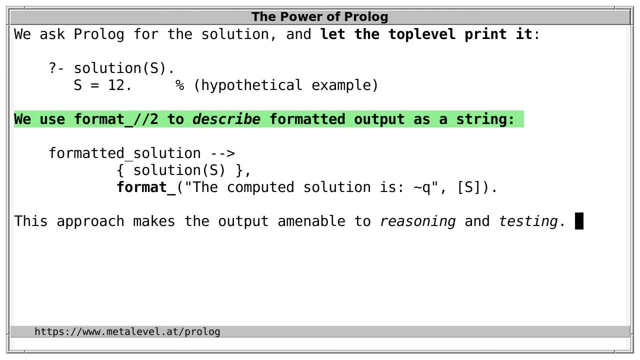 because the output is now amenable to reasoning and, in particular, to testing. So, for example, we can ask what is the list of characters s that is being described, And the top level automatically shows the answer. However, we see here that the string is truncated. 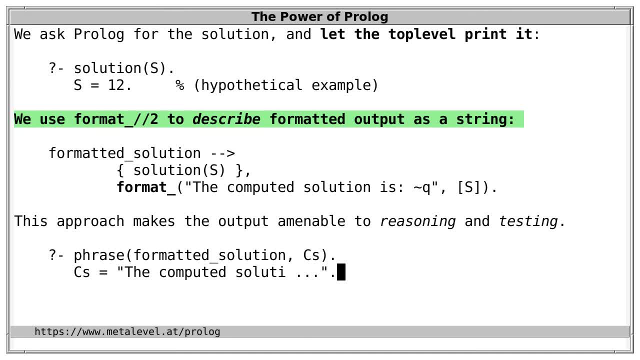 And we'd like to tell the top level to print it fully. However, in this case the query has succeeded deterministically, so we had no chance to interact with the top level, So we'd like to manually introduce a choice point to get this interaction. 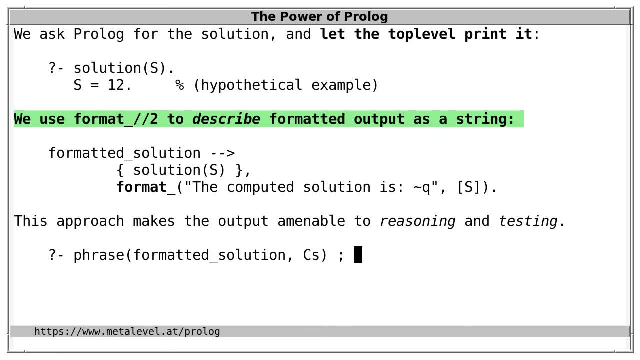 Now, how do we introduce a choice point? Certainly by introducing a choice, So, for example, with a disjunction, And then one may be tempted to use any predicate that first comes to mind, such as true. However, that would distort the truth of the goal. 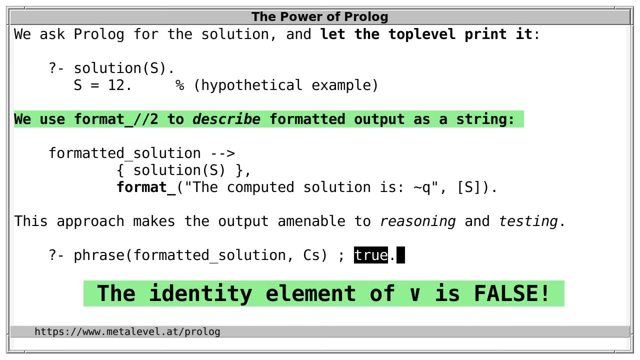 because the identity element of disjunction is not true but false. So we can use false here. And when we post a query, we can now interact with the top level And for example, in Scriapolo we can press W to write the entire string. okay, 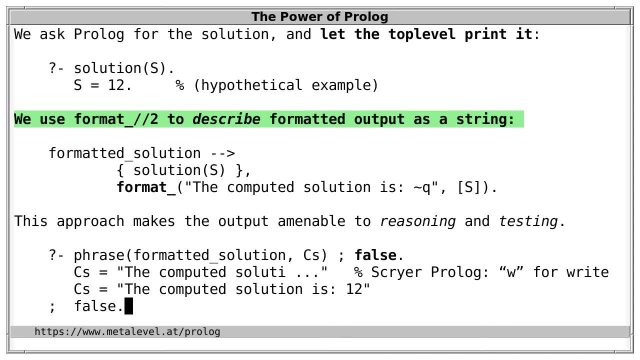 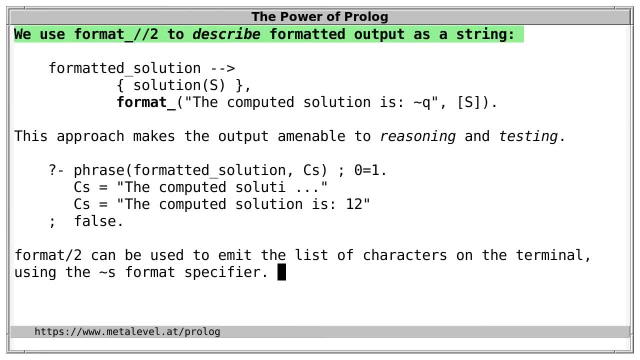 And on backtracking we get false, That is, there are no other solutions And we can make this a bit shorter, like this for example: And again we press W here, as before And when needed, the predicate format. 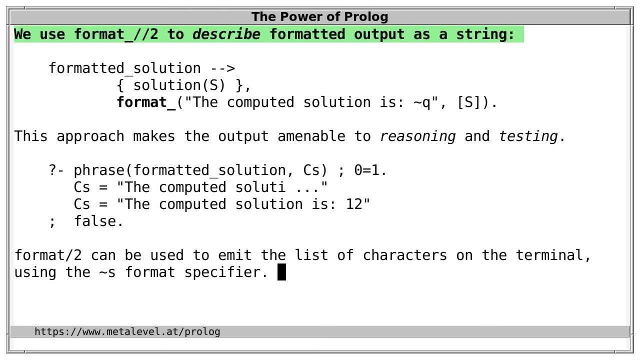 can be used to actually write this list of characters on the terminal with the S format specifier, which stands for string. So we would first ask for the list of characters Cs and then say we emit a list of characters, namely Cs, And so we get these characters as output on the terminal. 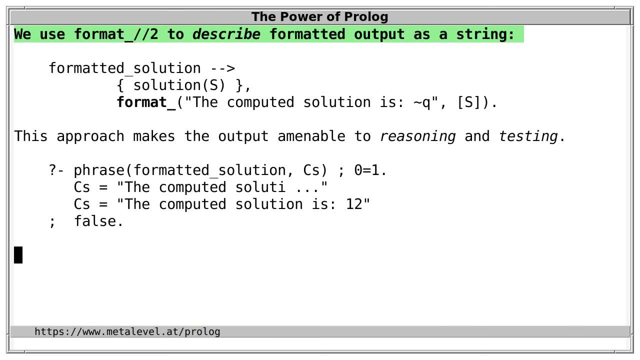 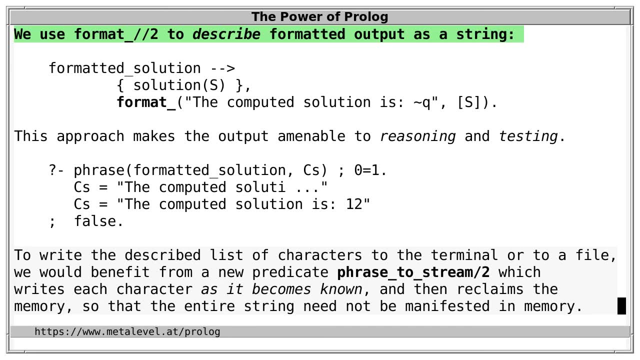 Of course, it's suboptimal that we had to manifest the entire list in memory, So what would actually benefit most from here is a new predicate, say phrase to stream, which writes each character as it becomes known and then immediately reclaims the memory. 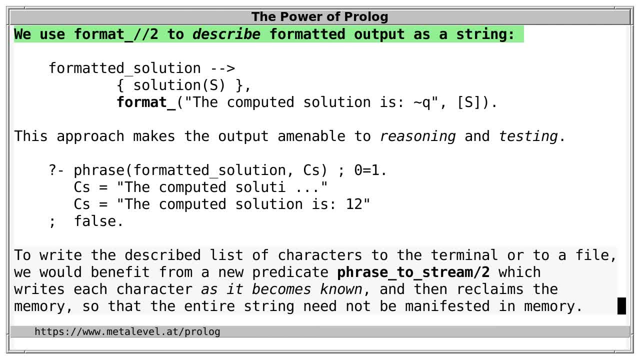 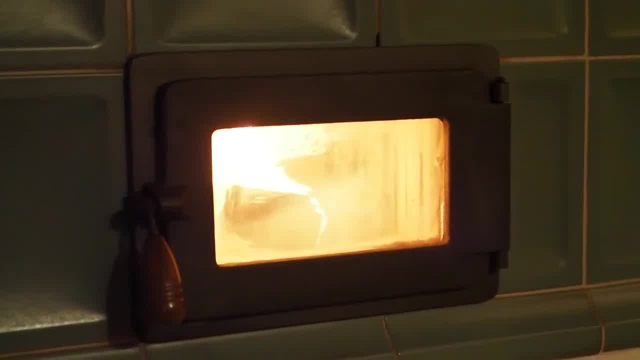 so that the entire string need not be manifested in memory, And Prolog implementers are, of course, highly encouraged to provide this predicate, because then we can make more of our list of code amenable to reasoning and at the same time achieve good performance. 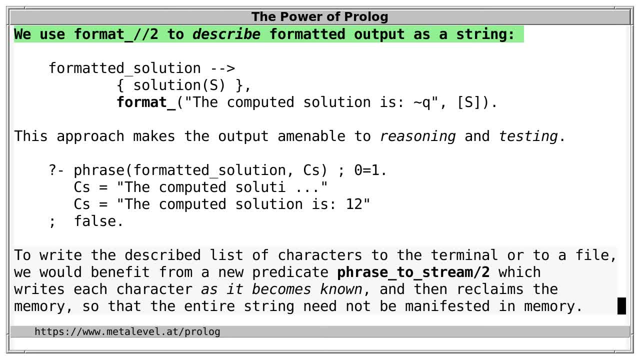 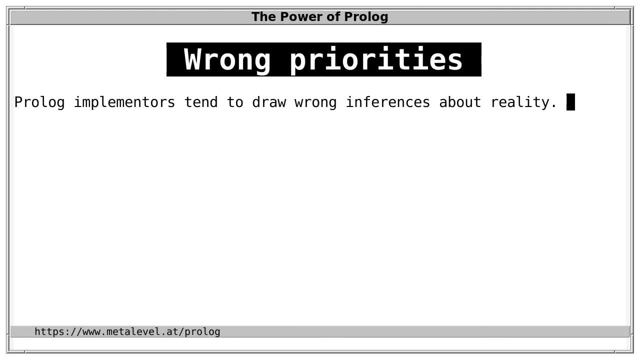 In this case, especially space efficiency. And speaking about implementers, they are also prone to anti-patterns because Prolog implementers tend to draw wrong inferences about reality. For example, if constraints are slow in a system, then implementers will tend to wrongly assume. 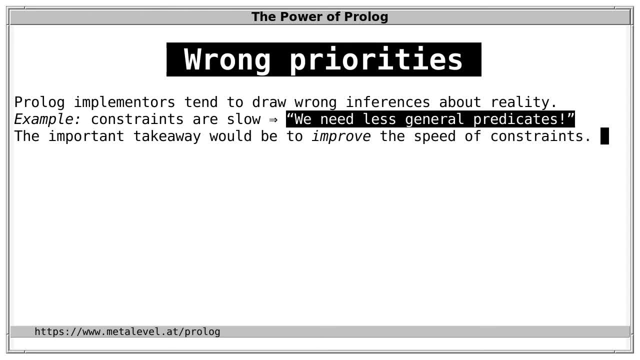 that we need less general predicates too, whereas the important takeaway would be to improve the speed of constraints, For example, with better interface predicates or better compilation and so on. And, of course, implementers are subject to a lot of pressure, for example. 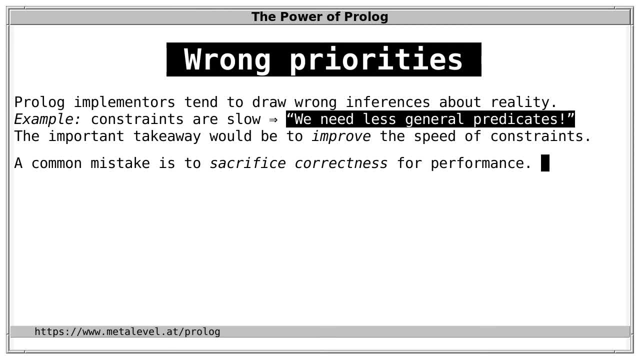 from publications and benchmarks about Prolog systems, which mostly measure performance, at least at the moment, Up to the point that implementers tend to sacrifice correctness for performance, Because if you ask customers: do you want a fast Prolog system, then they tend to respond yes. 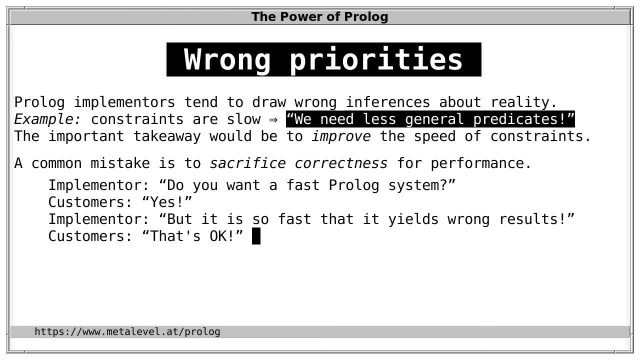 And even if it's so fast that it yields wrongly, it yields wrong results. Yes, that's okay. So customers should also think about what they actually need from a Prolog system, And personally, I think implementers are well advised to provide building blocks that let us write. 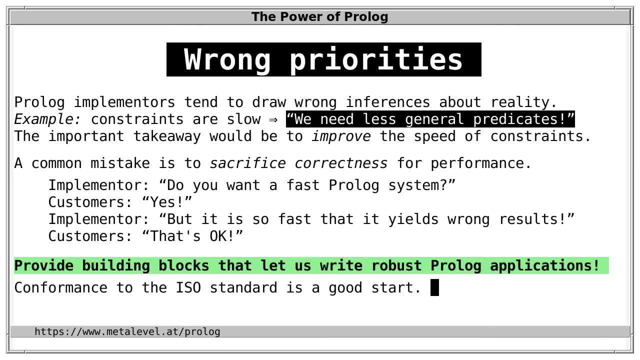 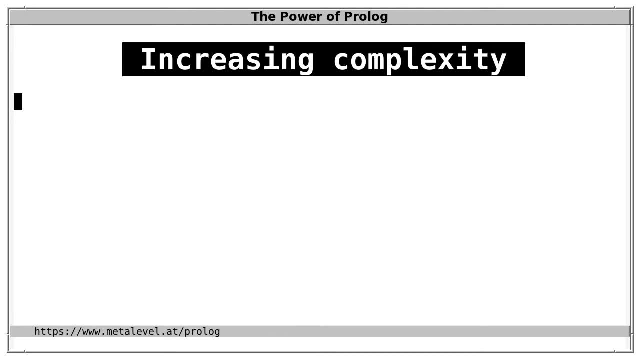 robust Prolog applications, starting with conformance to the Prolog ISO standard, then an efficient representation for strings, a convenient interface for attributed variables, reliable constraints, and so on. Another example or consequence of wrong priorities is when implementers increase complexity instead of decreasing it. 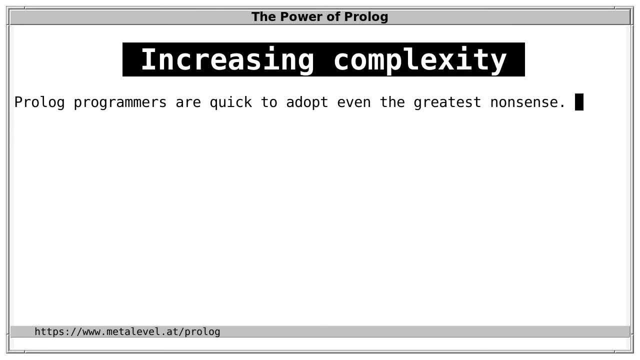 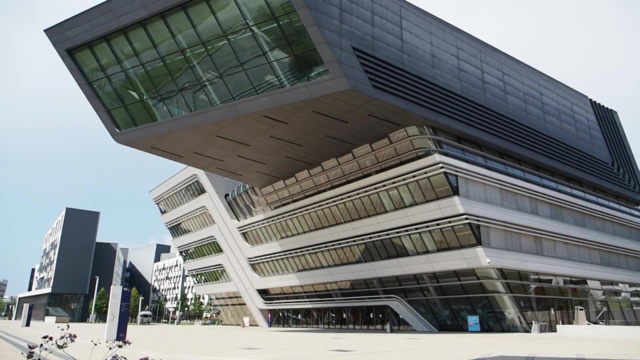 And this can happen quite quickly because Prolog programmers are quick to adopt even the greatest nonsense And therefore when an implementer comes up with a bad idea, then programmers often simply adopt it instead of resisting it. So popularity is no reliable indicator. 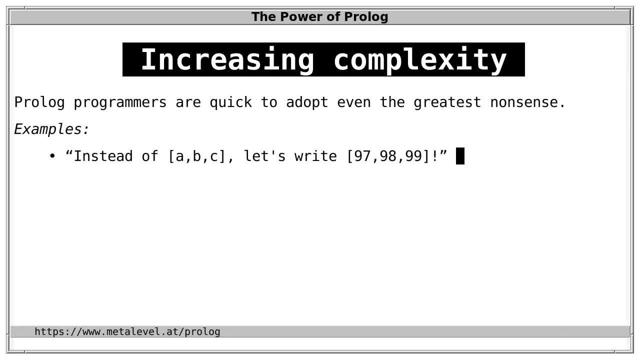 of quality and style. For instance, suppose I say: let's forget lists of characters and instead write characters using the ASCII codes. Then Prolog programmers, especially from Edimpro, will adopt this easily. Or even more extremely, let's forget lists and use a new data type. 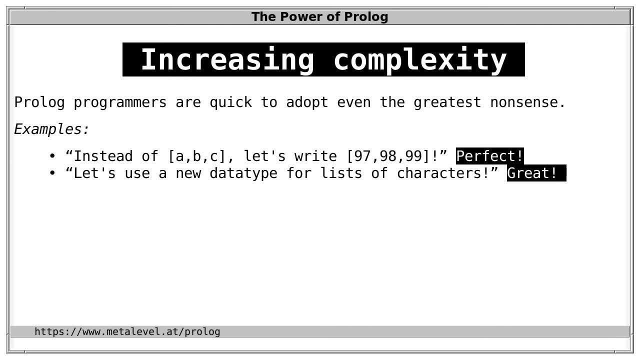 for lists of characters, Then Prolog programmers will also adopt it. Another such idea is, for example, to say: let's make write canonical. no longer emit the canonical representation of a term, but something else- Yes, of course. Or what about deviating from the standard entirely? 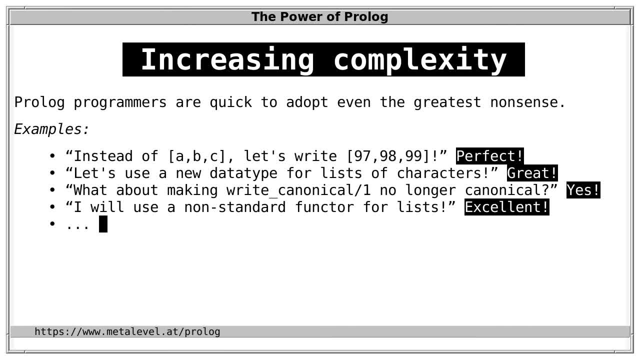 and using a different functor for lists Perfect right And so on. And I'm not pulling your leg here, because all these examples have actually occurred in the history of Prolog And some of them have set Prolog systems back by many years, if not decades. 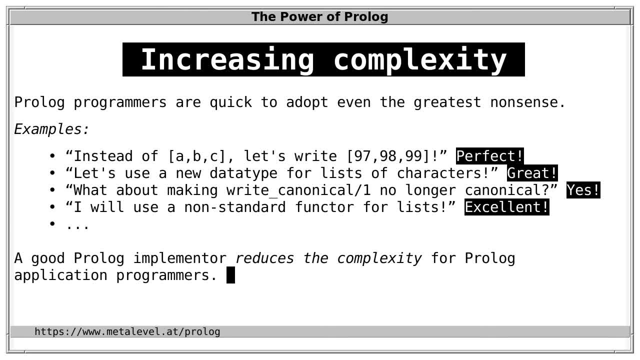 Whereas a good Prolog implementer always tries to reduce complexity for application programmers. For instance, we already have many predicates and also DCGs for reasoning about lists And therefore strings should be lists And to make them easily readable, they should be lists of characters. 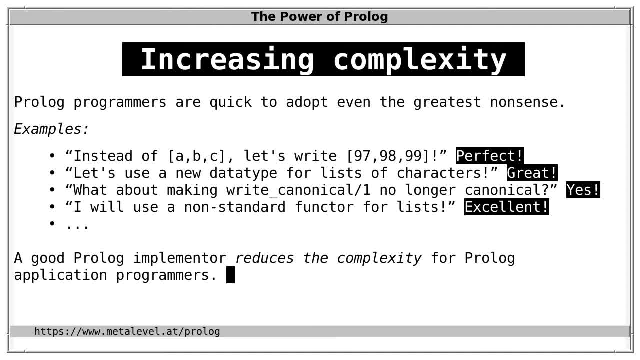 not integers, And if I want to print them canonically, then I should get the canonical representation of lists and so on, Because Prolog code should be simple and elegant and implementers should be committed to making this efficient, So the burden should be on the implementer. 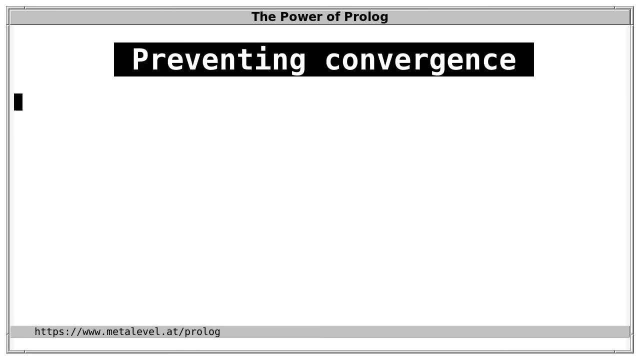 not on application programmers. Another example of increasing complexity is preventing convergence of Prolog systems, Because also here implementers are quick to adopt bad ad-hoc mechanisms which only cement the differences between systems. For instance, suppose I want to make Prolog code. 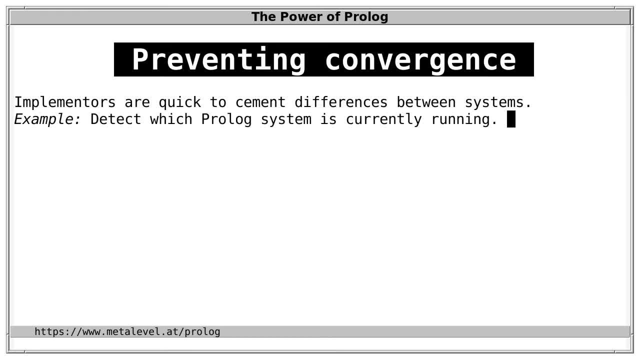 portable between systems. So the answer is easy, right, Simply provide a way to let me detect which Prolog system is running. However, the notion of dialect is alien to the Prolog standard. The standard only knows different degrees of conformance. 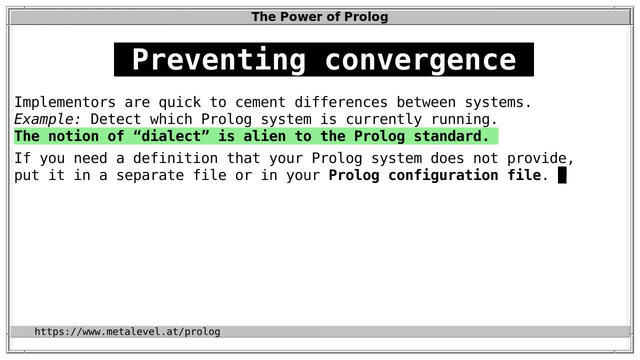 not different dialects, And we of course still aim to for convergence. So we want to write our code as if there were only one Prolog system And we don't want to make the code itself depend on any specific system, Because what if a new system comes up? 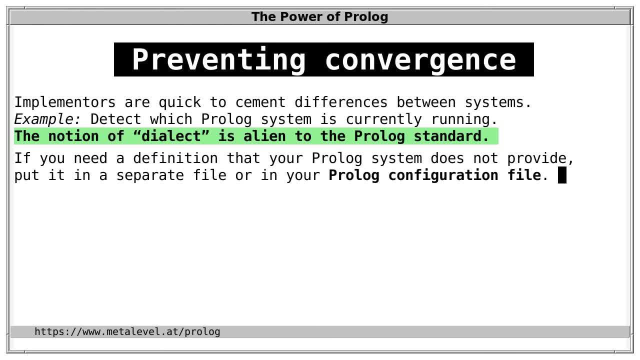 Ideally that should automatically also work right, So we don't want to tie the application to only a subset of systems. Therefore, instead of checking for which Prolog system is running, it's better to check for features Or to create separate files. 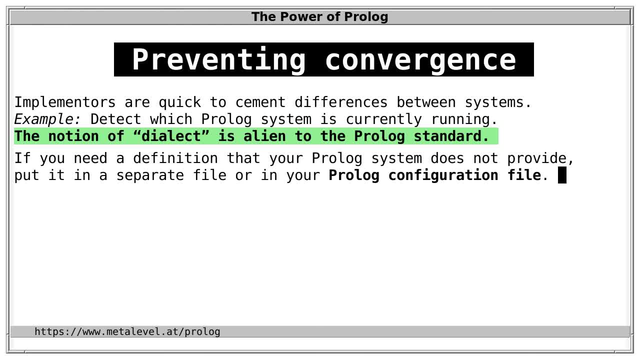 with system-specific definitions Or to make the necessary adjustments in our system's initialization file, And then we can simply load the definitions we need. For instance, when using Scrire Prolog, we load the application code and maybe some Scrire-specific definitions. 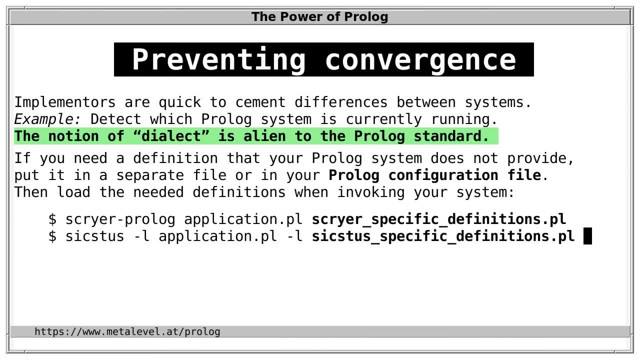 And for Sixtus we also load the application code and maybe some Sixtus-specific definitions, And likewise for other systems, Because in this way we are making a clear statement to implementers: We as application programmers will not carry the burden. 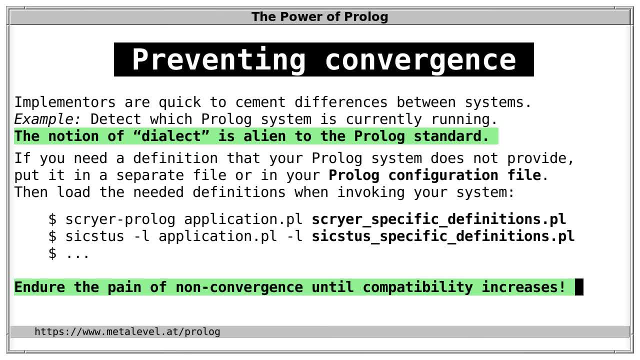 of plastering our code with additional checks. We are willing to tolerate maybe some additional compatibility definitions and also to provide them, But we are not making our code ugly just because the implementer has adopted bad practices. And lip service from implementers is not enough. 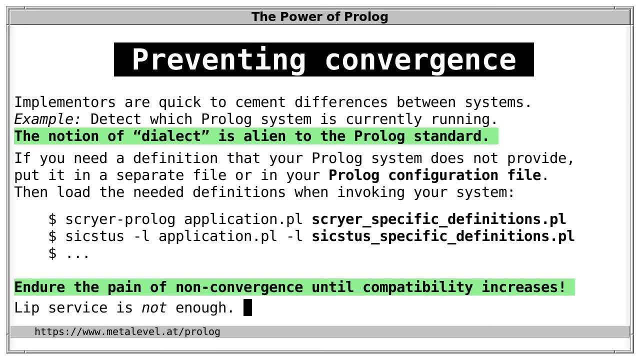 Because implementers are quick to say: we should all sit together and decide on compatible features and so on. So, yes, we wait for them to do it. And also, you are not only the messenger if you say: well, that's just how it is. 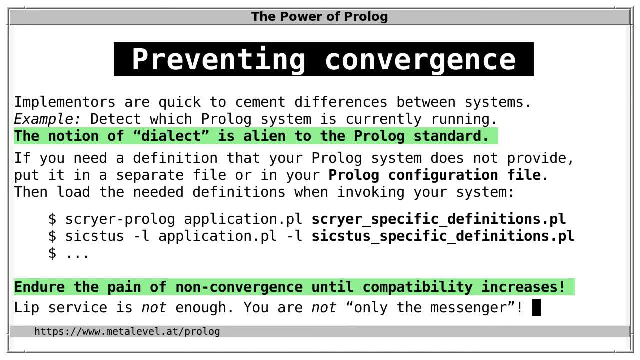 There is this incompatibility and so on, Because you are not just a messenger if you are choosing what to propagate, And you are especially not just a messenger if you personally benefit from incompatibilities between systems, For example, if you are selling or providing. 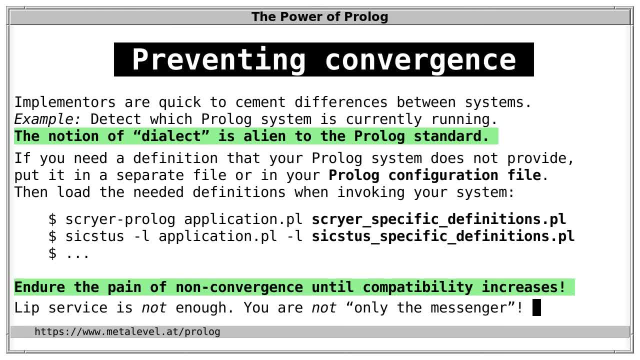 a framework that itself acts as a compatibility layer, right? Because then it's in your own interest to prevent convergence between systems, Or at least it has the appearance. So we wait it out, instead of adopting practices that only cement the difference between systems. 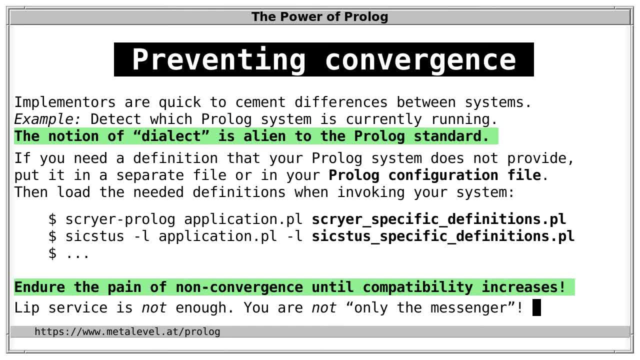 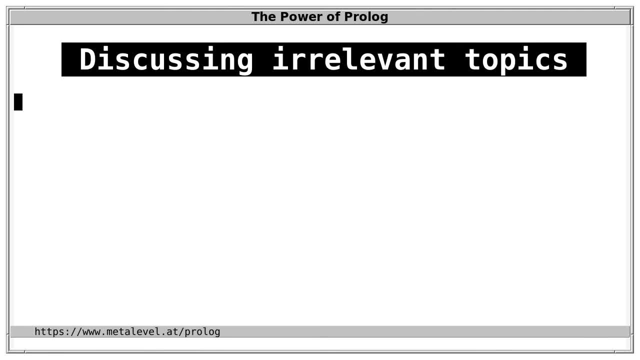 And, in the interest of convergence, we are not testing which system is currently running. Now, from programmers and implementers, on to prologue instructors. A typical prologue instructor may have about 10 two-hour slots to teach prologue, Maybe a bit more, maybe even less. 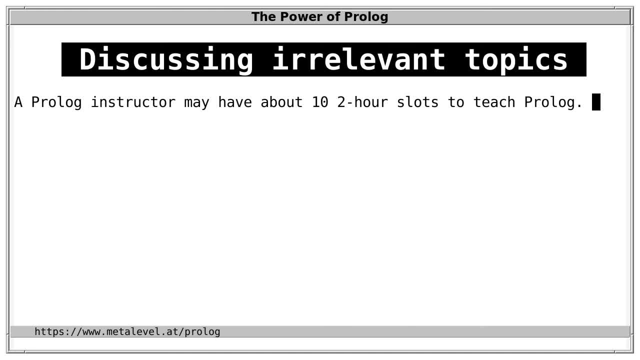 And prologue instructors tend to spend a lot of the little time they have on irrelevant topics. For instance, how much of this time do you want to invest in explaining cut? And how about not only explaining it but also complicating it? For example, what about making up? 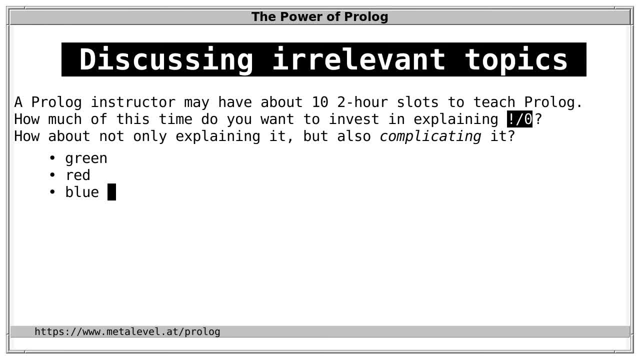 our own categories of cuts: Ring cuts or red cuts or blue or even grue cuts. I mean, seriously, is this how we want to spend our time With an elaborate litany of completely made-up concepts? No, of course not, because our goal 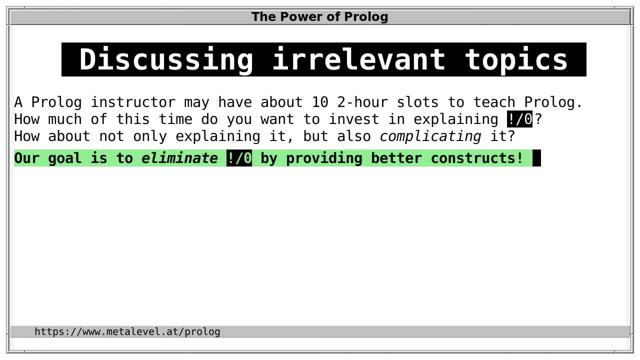 is to eliminate cut by providing better constructs. Or, as another example, take proof trees. What are we supposed to do with a proof tree? Should we read it? So I really wonder which prologue instructor has time to introduce an additional formalism too. 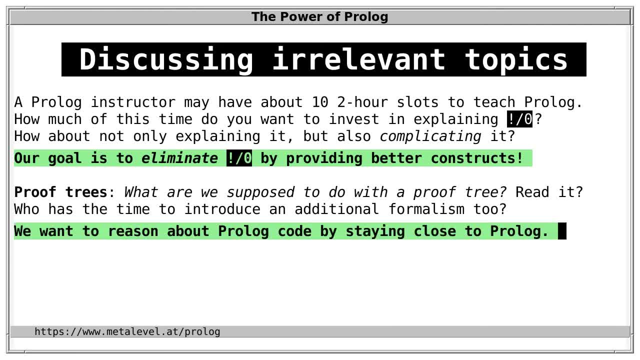 A prologue instructor should teach prologue, and we of course, want to reason about prologue by staying close to prologue, Because if you're using a different formalism, then who can tell whether, and to what extent, this actually has anything to do with the given prologue? 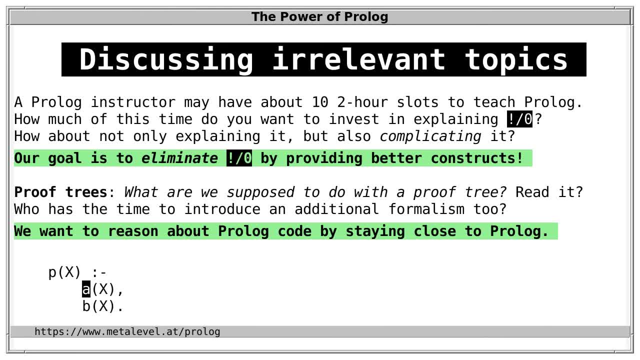 program. And a good way to reason about prologue code is to think in terms of generalizations and specializations. right, For instance, we can generalize away a goal And we should make this reasoning possible. So a prologue instructor should teach constructs. 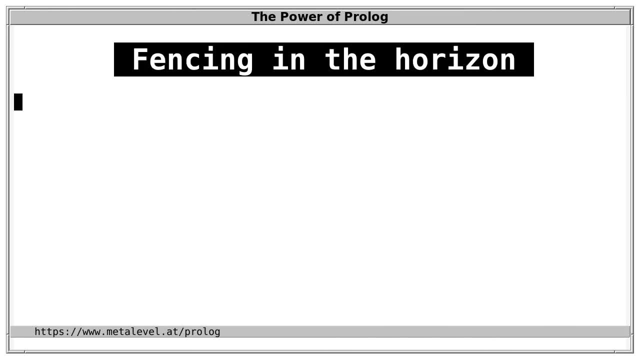 that admit this reasoning. And all these antepatterns have one thing in common: The fence in the horizon. I don't mean the fence in the horizon, but the fence in the horizon. So the limit, the horizon, Because the overarching commonality. 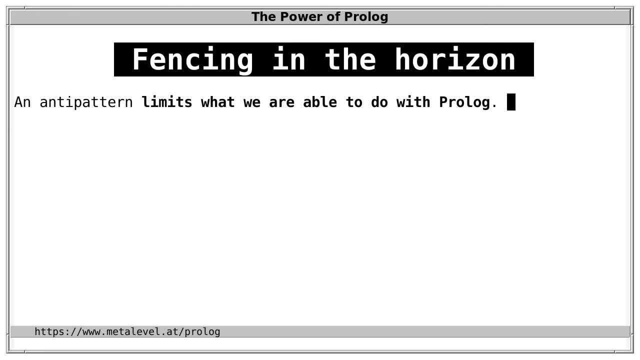 of all these antepatterns is that they limit what we are able to do with prologue, And destroying logical properties is the most common antepattern, Mostly by teaching outdated and problematic language constructs. Another antepattern is to not teach enough constructs, Maybe. 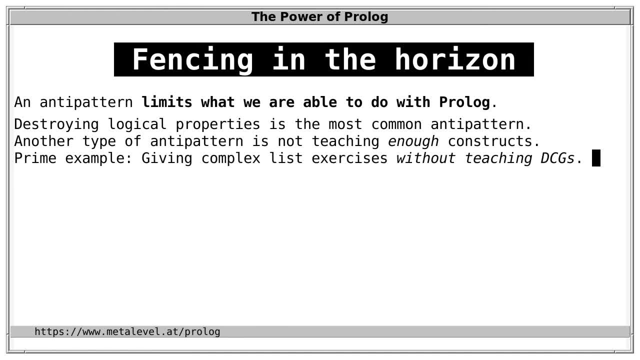 the prime example for this is to give complex list exercises without teaching DCGs, Because many relations over lists are very easy to describe with DCGs, Such as relating a list ls to its last element, l, Which holds if and now. we use a DCG to define the. 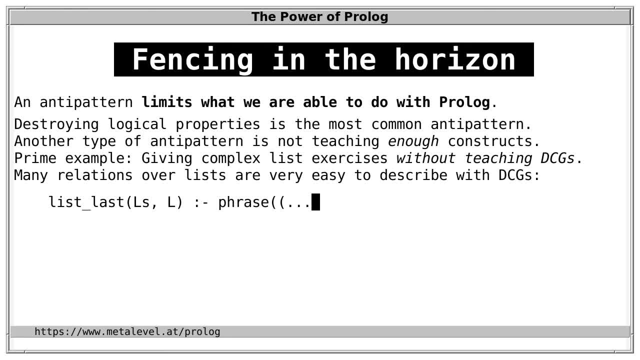 relation. So the list we are describing has the form dot, dot, dot, denoting any list at all from library DCGs, and then the last element, l, And if ls is of this form, namely anything at all followed by l, then the relation holds, So l. 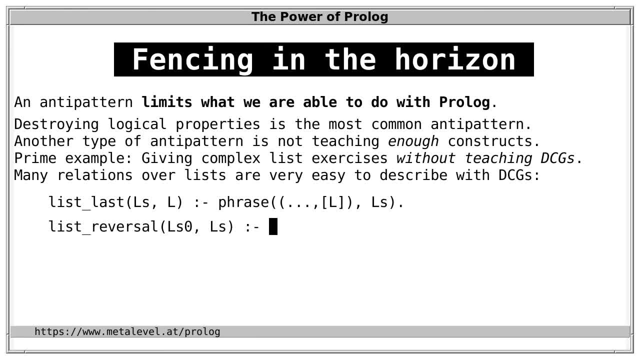 is the last element of the list ls, Or as another example relating a list ls 0 to its reversal ls. We can also easily describe it with a grammar and I leave it as a challenge. And speaking of list exercises, flatten is not a good exercise at all. 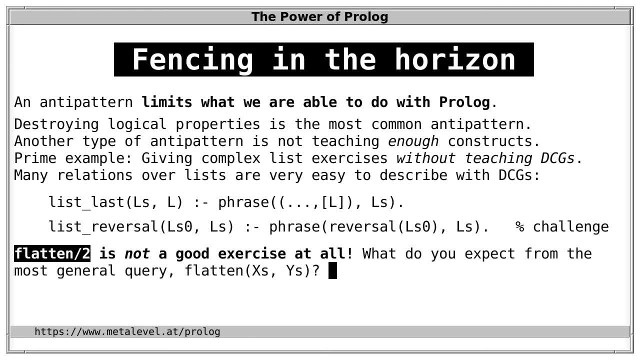 Even though it's often given to students, Because what do we expect from the most general query where we ask: for which lists does it hold? in general, Is this a monotonic relation, And can we implement it so that it preserves monotonicity? 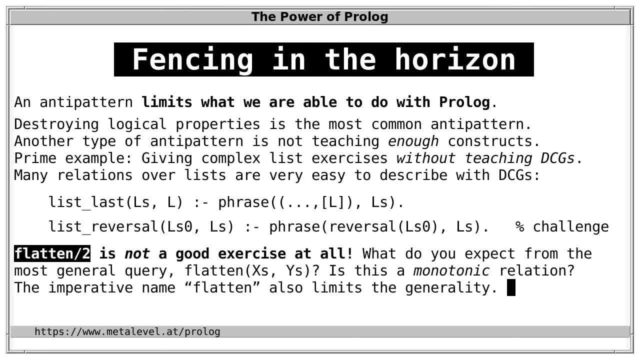 And the name flatten is already problematic in itself because it's an imperative, And thinking about a relation imperatively already limits the generality and what we can describe with it. So limiting the horizon is also a common anti-pattern and we want to do the 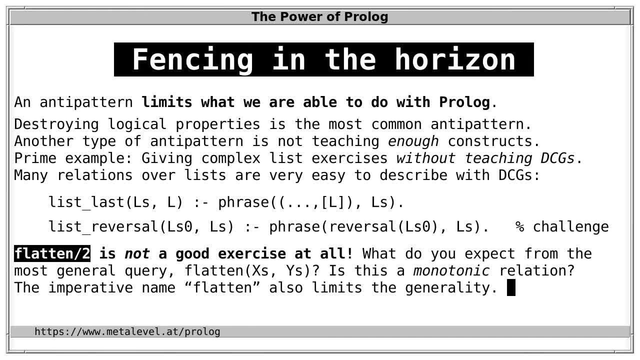 opposite. We want to use Pollock to its fullest potential, And for this we keep to its pure monotonic core, Because in this way we can reason logically about the code and we can easily analyze it, Run it with different execution strategies and so on. 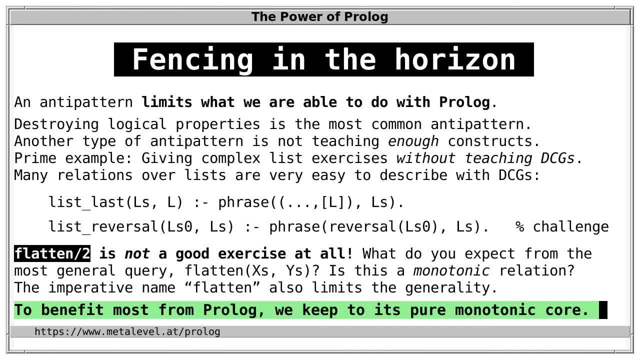 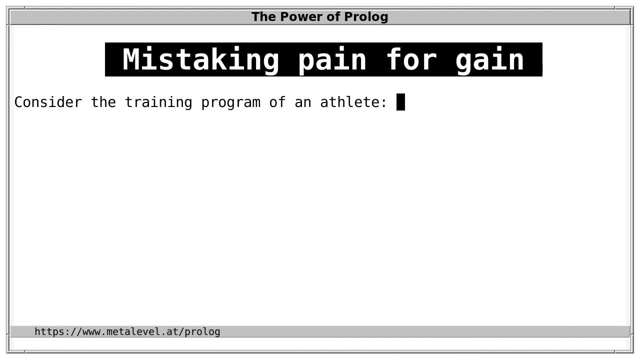 Now you may say, wait a minute. Am I not also fencing in the horizon by advocating that only a subset of Pollock be used? So am I not also limiting what we can do with Pollock? Well, to answer this, consider the training program of an athlete. 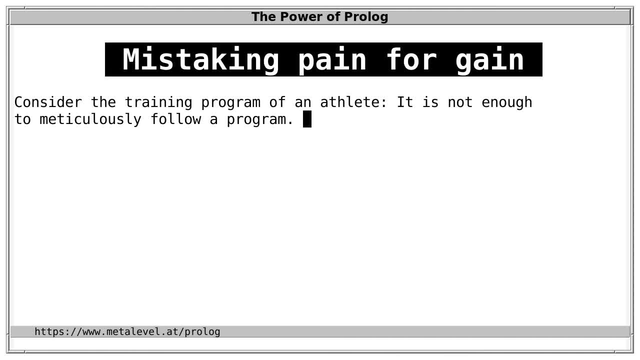 It's not enough to meticulously follow a program. That's only a necessary condition for a top athlete, Because the training program itself must also be well designed and tuned. And not only that, because recovery phases are at least as important as the training. In a sense maybe even more important. 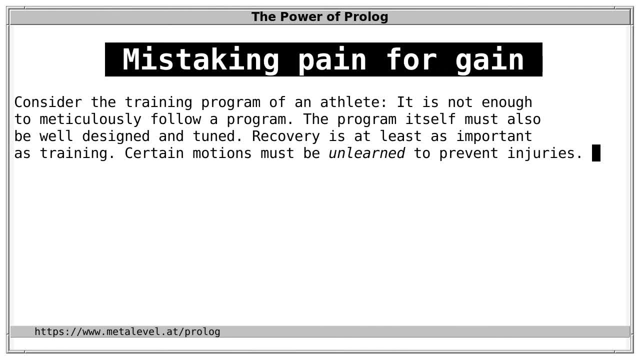 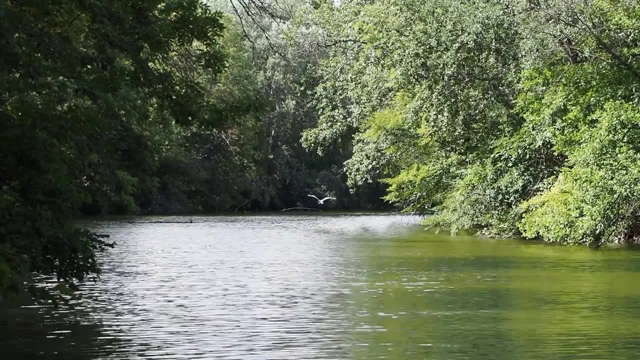 And also certain movements must be unlearned, to prevent injuries or to maximize power or to increase stamina, to eliminate redundant motions. And indeed you'll find that in many disciplines an important factor for success is to make only the necessary moves. And if you're training hard, 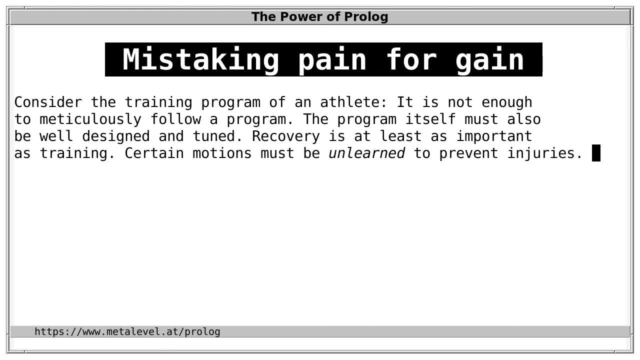 it may be painful, At least a bit, Because it may be tough to endure, or your muscles will ache and so on, And if you train effectively, then you may consider the pain worthwhile, Because you're also gaining something Such as more endurance. 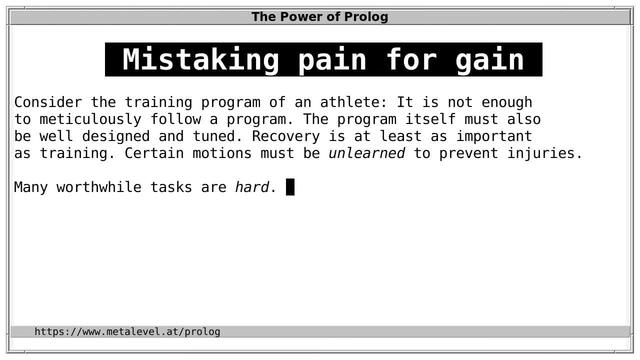 more power, more mental strength and so on. And there's no doubt that many worthwhile tasks are hard. For example, learning a new sport, an instrument or a language and so on can be quite hard and even painful, And also worthwhile, Yet excessive hardness. 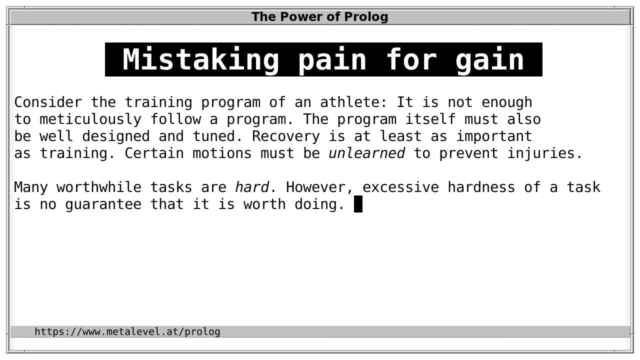 of a task is no guarantee at all that the task is worth doing, Because many things that are hard are also pointless or even counterproductive, such as, for example, learning without enough sleep and so on, Or playing an instrument with a wrong technique. And I mention these examples because in the 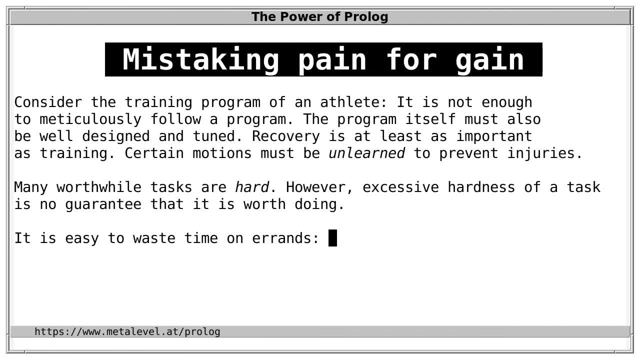 prolog world, it's easy to waste time on pointless errands. For instance, implementers sometimes put effort into deviations from the standard And programmers often start catering to the machine instead of talking to implementers, so that the underlying system is improved for everyone at once. 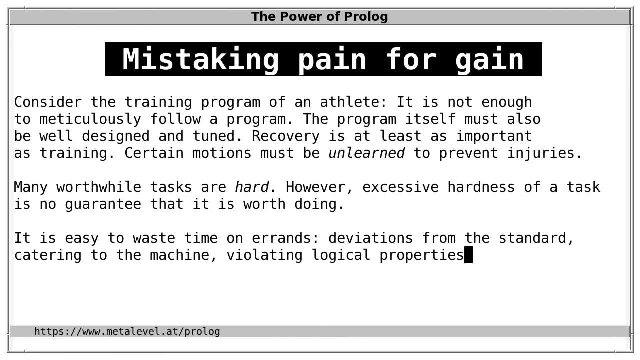 Or, as mentioned, a lot of time is wasted on constructs that violate logical properties and so on. So these tasks may be hard right, And they're also counterproductive, Because we want to make our tasks as easy as possible so that we can do more with prolog. 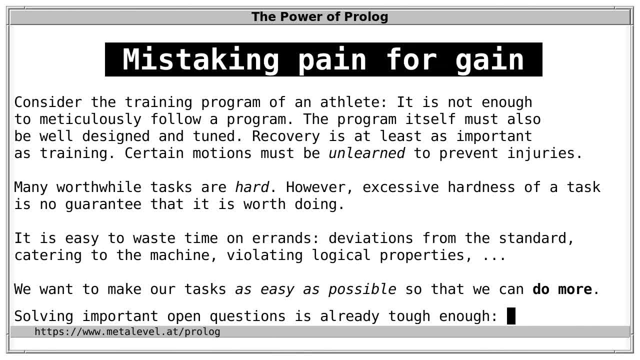 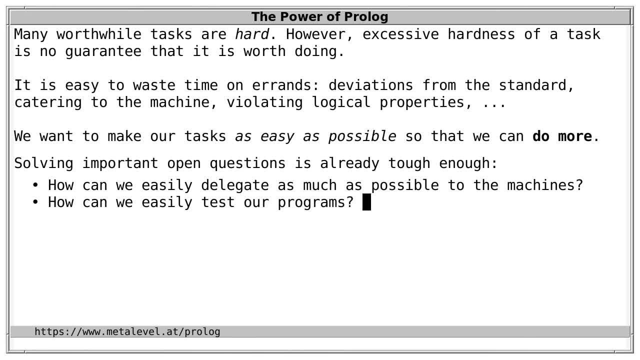 And there's no need to make this harder, because the challenges are already tough enough. For instance, how can we easily delegate as much as possible to the machines? How can we easily test our programs? How do we ensure that we can easily reason about our programs? 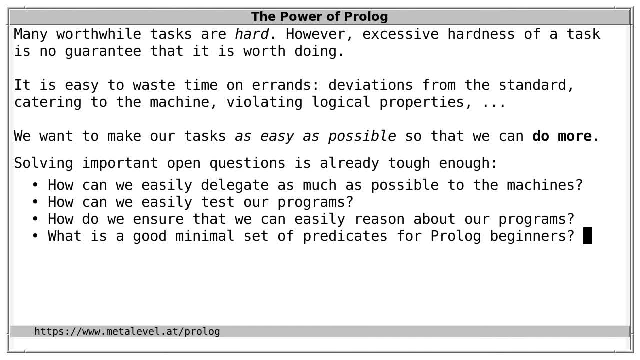 What is a good minimal set of predicates for prolog beginners, For example? do we really need the predicate format And wouldn't it be better to provide format underscore together with phrase-to-stream, which is very general? And which additional language constructs are needed, For example? 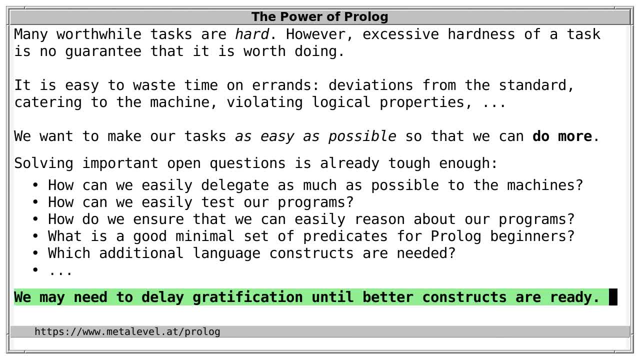 what about list comprehensions And so on? And we may need to delay gratification until better constructs are ready. This means that there may be programs that we can't write satisfactorily at the moment Because we don't have the right billing blocks available- at least not 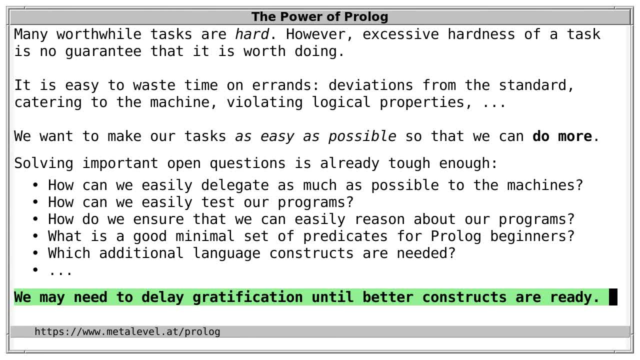 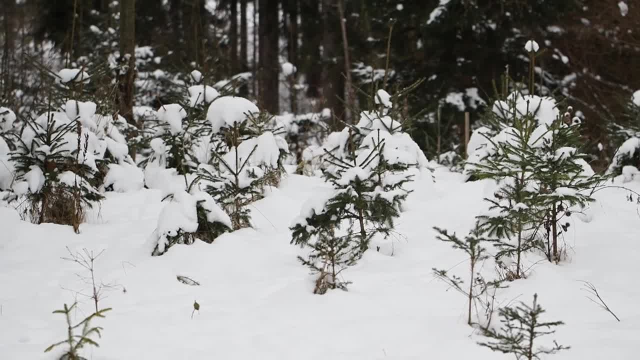 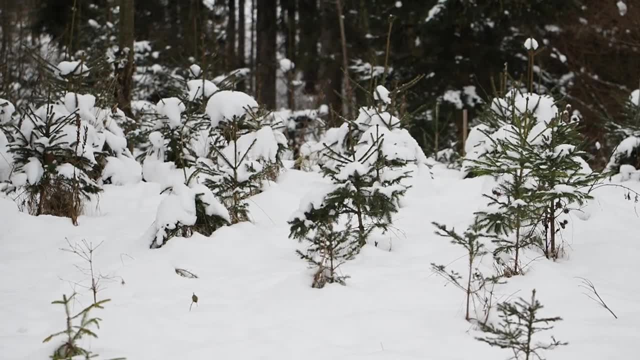 yet- And this only means that we have to keep looking for better constructs- We hunger ourselves up Like trees, Because in a healthy forest the young trees don't get much light And therefore they grow slowly And therefore the wood becomes strong And 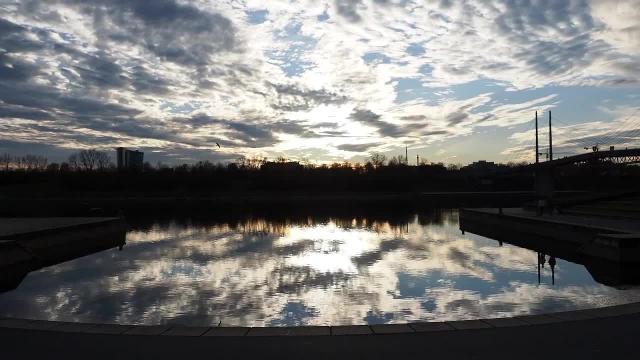 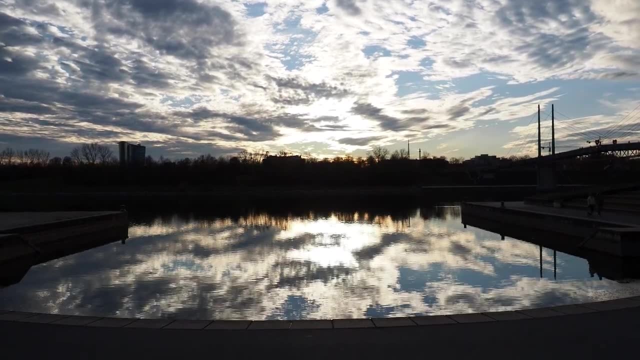 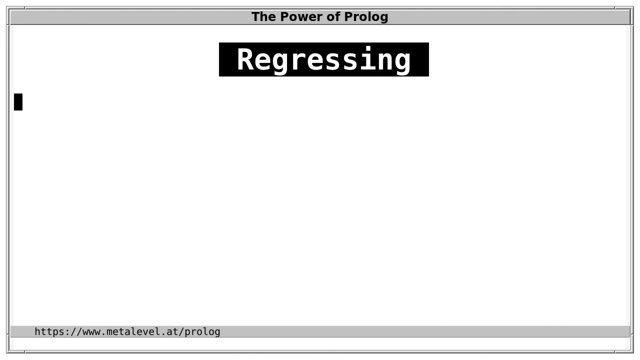 we accept nothing but the best. So we truly want the best constructs, not the hardest or most painful ones. Writing elegantly, programs should be easy, As easy as possible, And finally, maybe the strangest anti-pattern of all, Namely regressing. 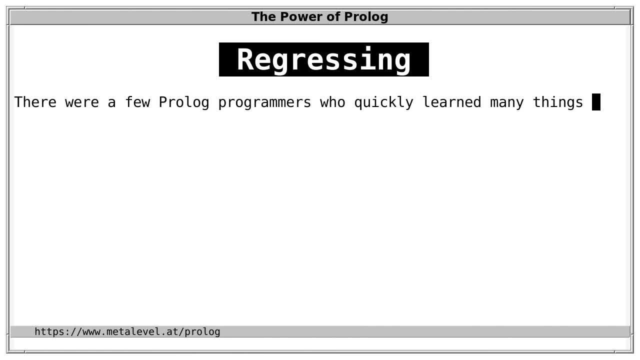 Because I've seen a few polar programmers- not very many, but still at least one or two- who very quickly learned many things and then regressed In the sense that they'd suddenly start recommending constructs that an experienced polar programmer will try to get away. 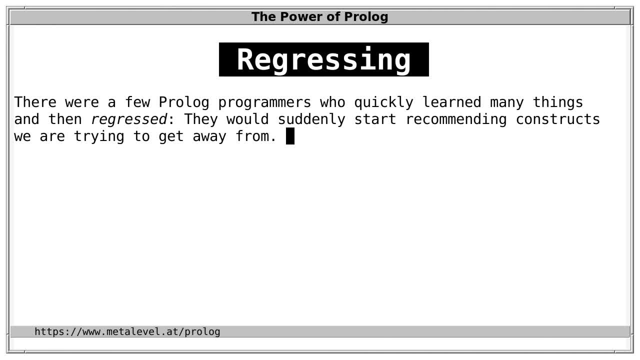 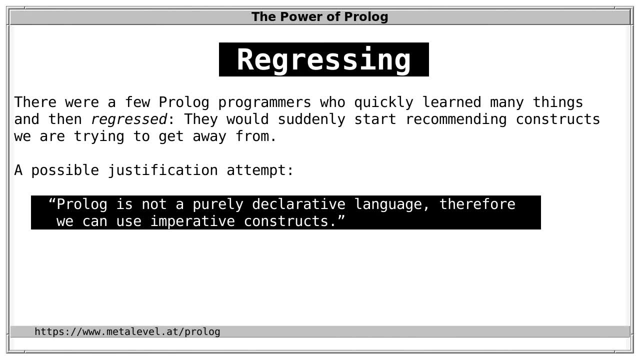 from Because they are too hard to use and reason about, And I don't know why such a regression happens. Maybe they internally try to justify it with. Prolog is not a purely declarative language and therefore we can use imperative constructs, But the reality 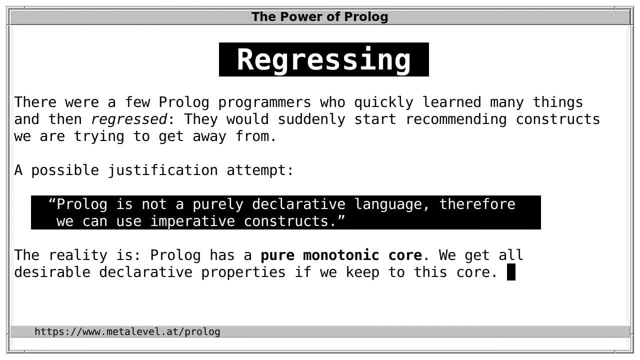 is that Prolog has a pure monotonic core And we automatically get all desirable declarative properties. as long as we keep to this core- And it's one thing to slip and occasionally maybe use a construct that destroys these properties- That's comparable to an athlete. 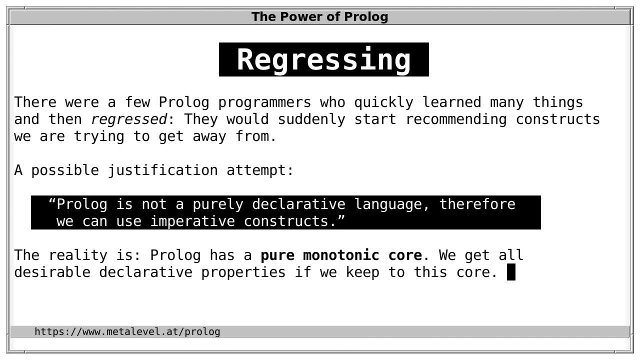 who falls and then immediately gets up again, But it's a completely different thing- and this is what happened here- to start running into an entirely wrong direction. And what's strange, in addition to this, is that the regressed users are often also the loudest. 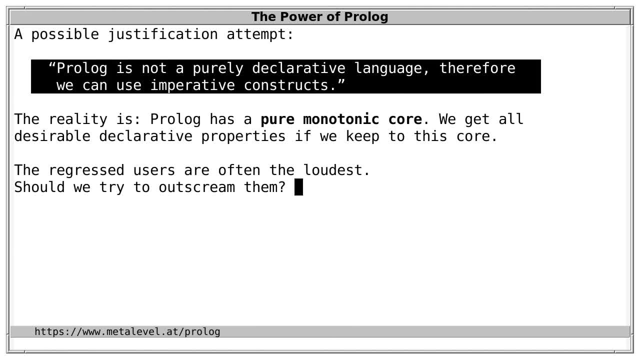 So they even advocate the regression, And we must decide now. Should we try to out-scream them? And personally I think no, because our task is to prepare a free Prolog system that has all desirable properties, guarantees and features with the goal. 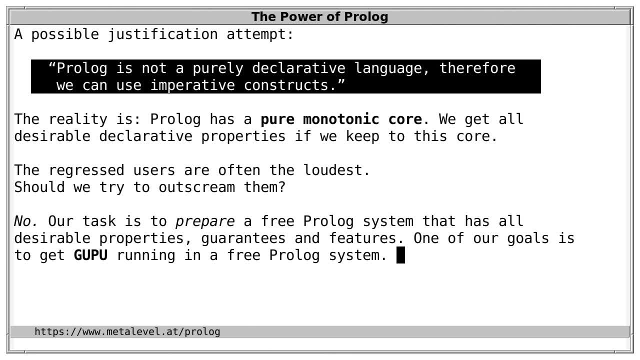 to run the Prolog teaching environment, GUPO, in a free Prolog system. Because GUPO will make the relevant arguments for us. Because GUPO first of all enforces the pure core and, second, shows what is possible. 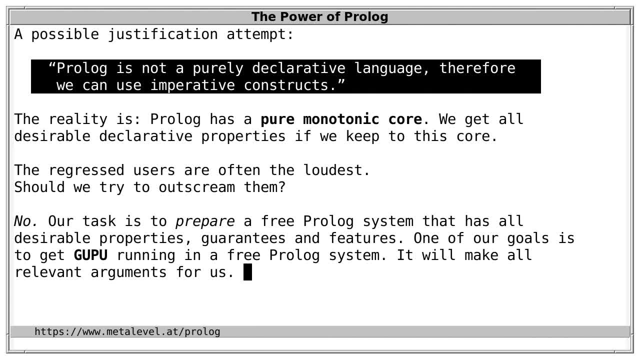 for example, termination analysis and so on, if we keep to the pure core. And importantly, GUPO makes Prolog education scalable Because we can run it for hundreds and thousands of students at the same time. So, to prevent regression, keep in mind that. 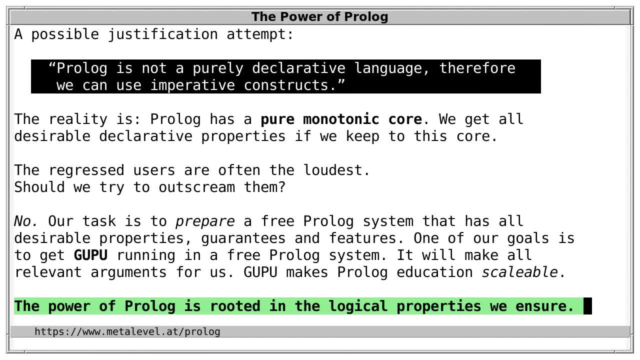 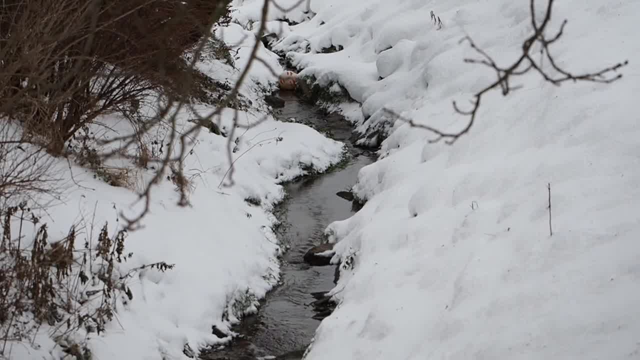 the power of Prolog is rooted in the logical properties we ensure, And if we violate them, then we can no longer depend on them, And then the core attractions of Prolog are lost.